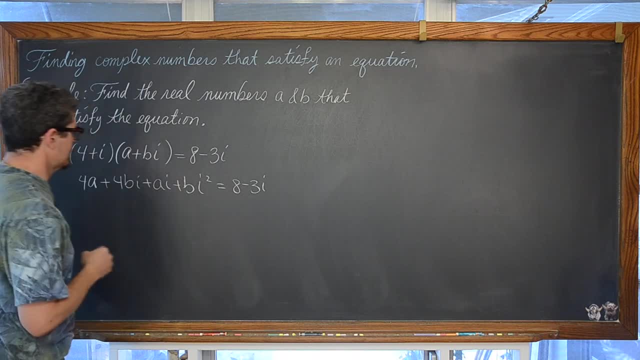 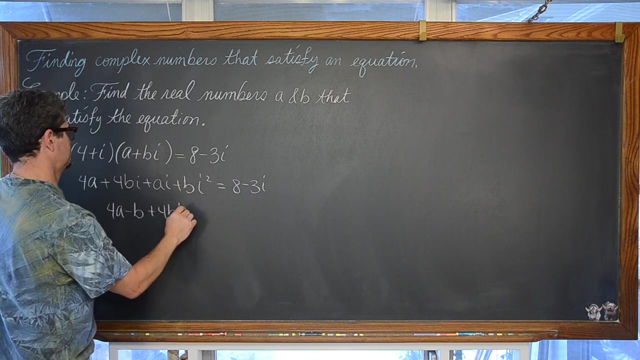 negative 1.. Therefore, i squared is equal to negative 1.. So this i squared is going to become negative 1, making this basically minus b. So we have 4a minus b plus 4bi plus ai is equal to 8 minus 3i. 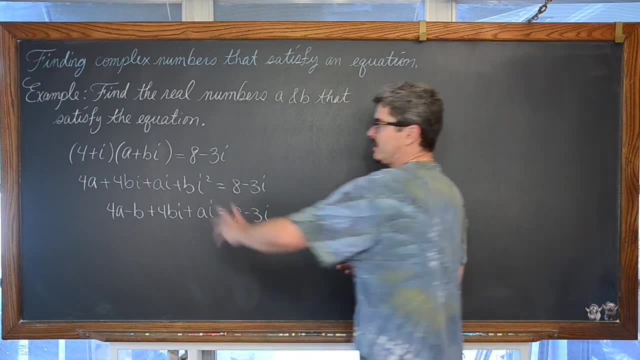 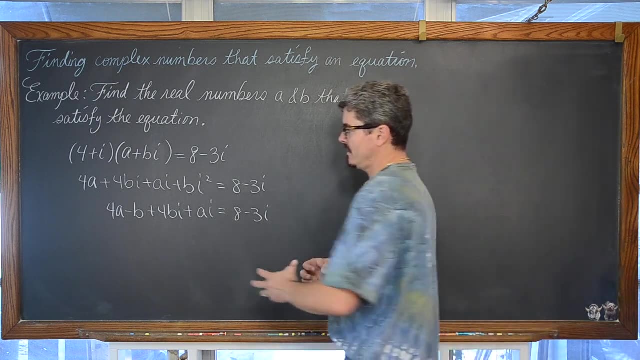 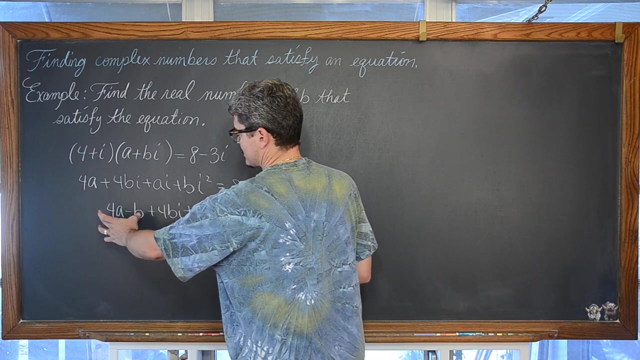 Subtitles by the Amaraorg community. now, if you look at the left hand side of this equation and you decided to distribute these two binomials together, then what you want to do is bring together, like i have here, your coefficients that are going to be the coefficients of a real value, in a sense. Well, 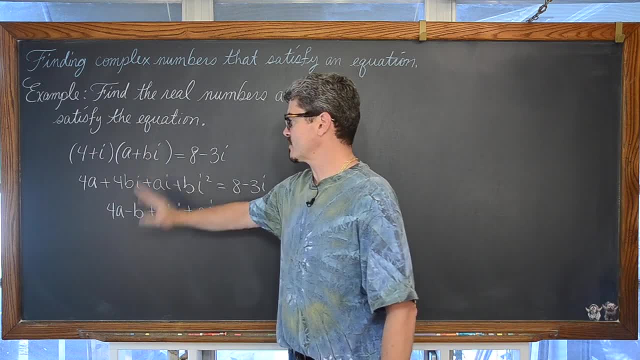 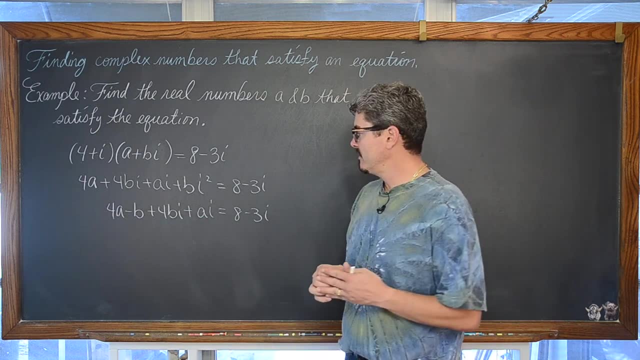 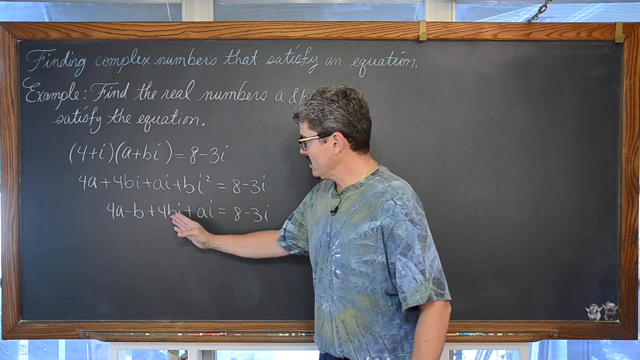 I am misspeaking here a little bit because kind of technically, b is a coefficient of our imaginary number or value of i. I am grouping together the terms that don't have an i in i in them, that are in themselves not a coefficient of an imaginary number. Here we have 4b times. 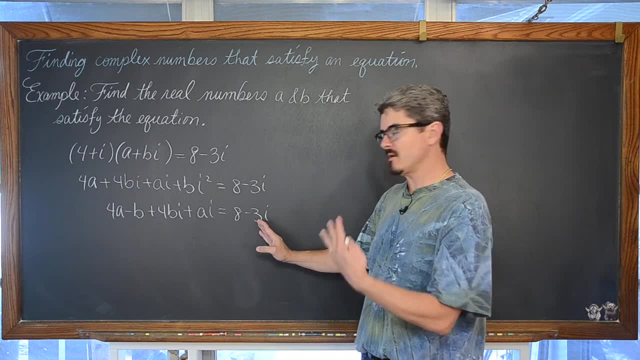 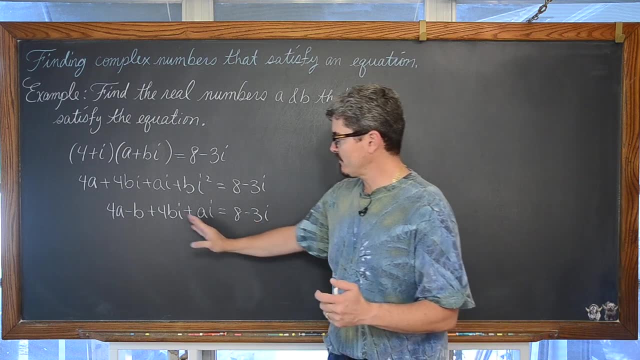 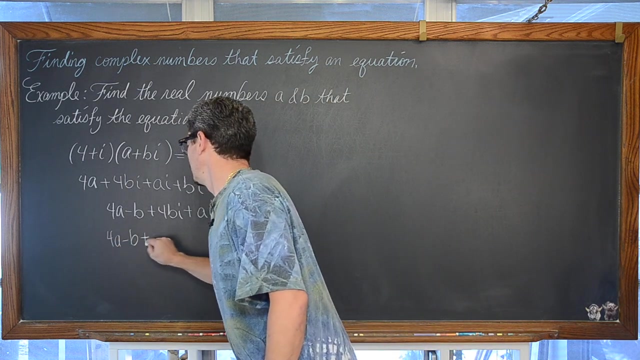 i plus ai and I want to match this up and kind of create an equation with the coefficient that i has on the right hand side of this equation, which is negative three. So I want to factor out our common factor of i from these two terms. So that is going to give. 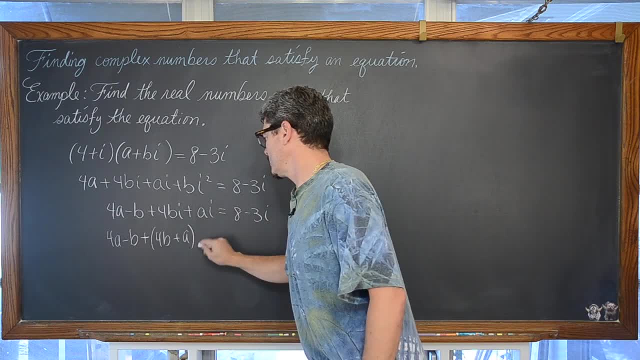 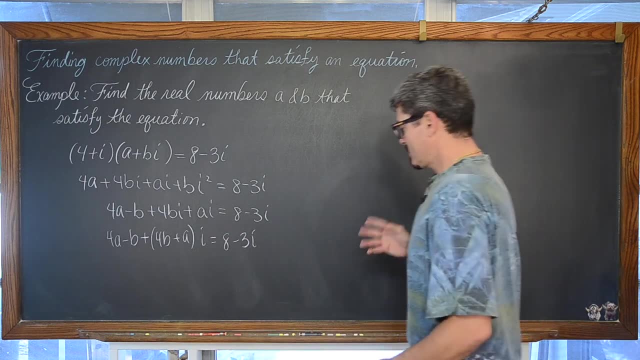 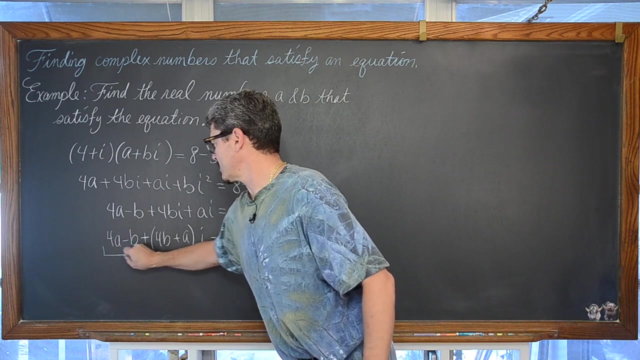 us a plus, and we have 4b plus a, which is a factored coefficient now of i, which is equal to 8 minus 3i. So we have this 4 minus b, which is slightly confusing because in our complex number b is the coefficient of i, It is the coefficient of our imaginary portion of our 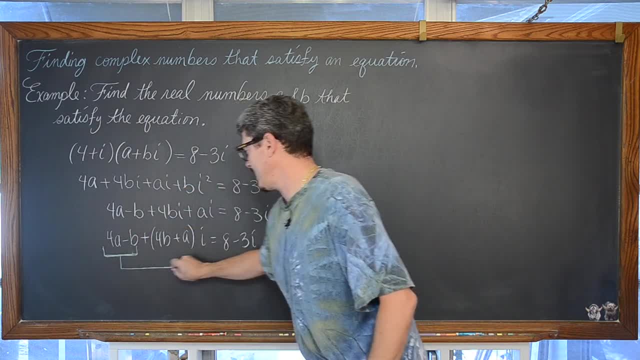 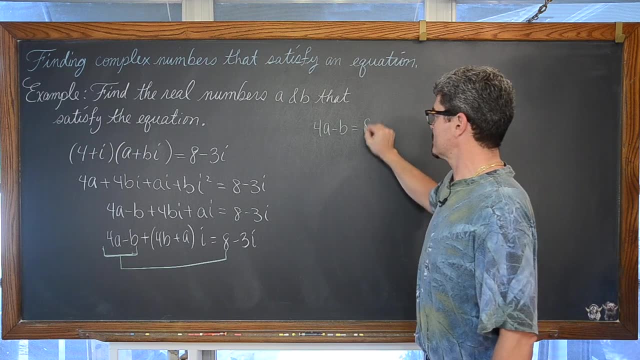 complex number, but right here b doesn't have an i with it, So this is going to be matched up with the 8. We are going to create a little equation with that and say that we have 4a minus b is equal to 8. Setting equal the real parts of the complex number, that is on. 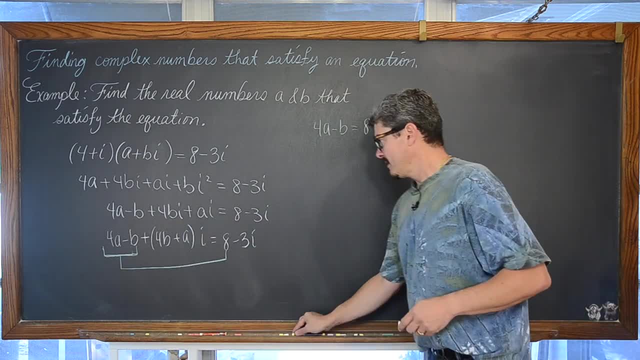 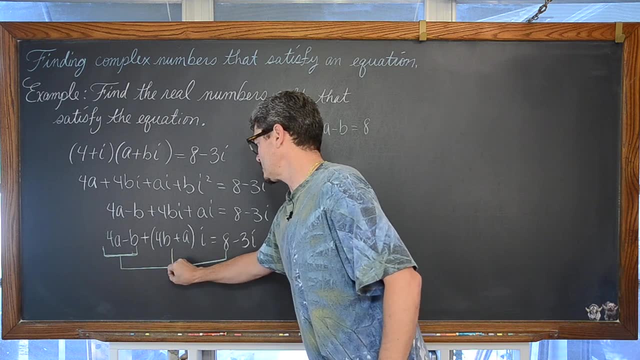 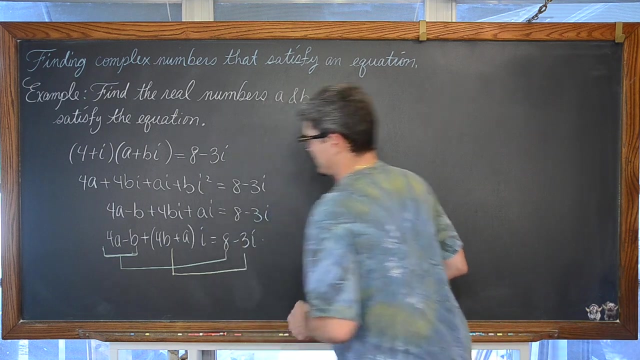 each side of this equation. Now we have a coefficient of i which is equal to 4b plus a. We are going to set that up to be equal to the coefficient of i on the right hand side of our equation. I am also going to turn this around because I am used to seeing the 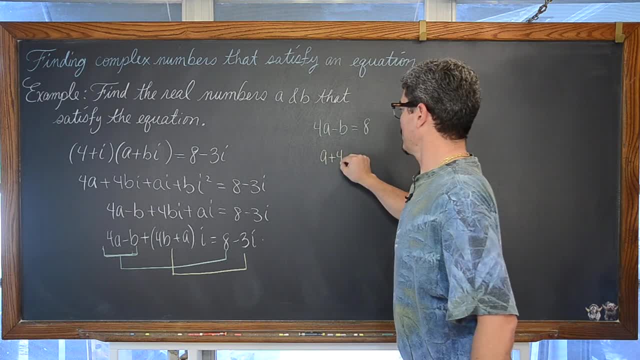 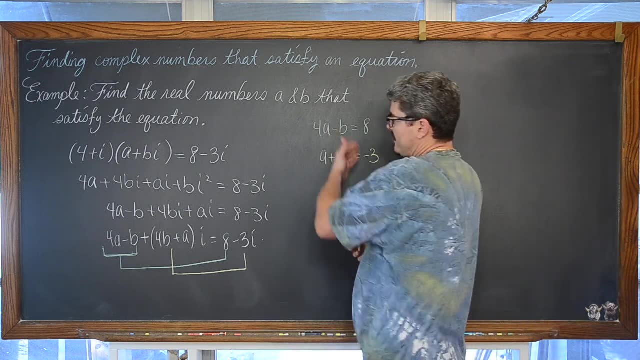 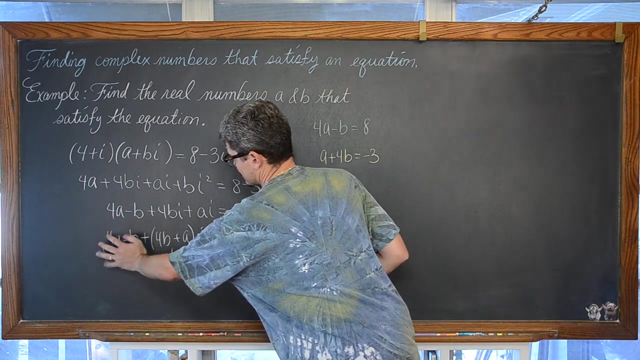 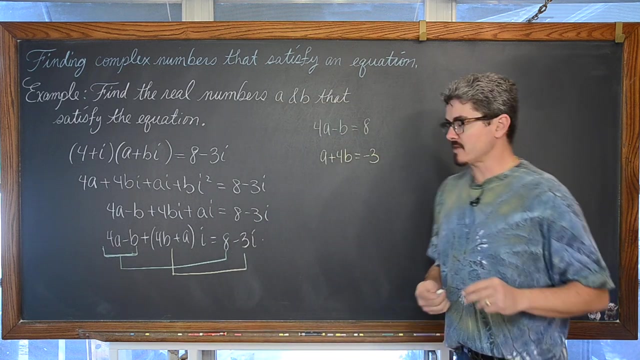 a first, We have a plus 4a for b is equal to negative three. Okay, so we now just have a linear system, a two variable linear system comparing the real portion of the complex number on the left to the real portion of the complex number on the right and the coefficient for i on each side of 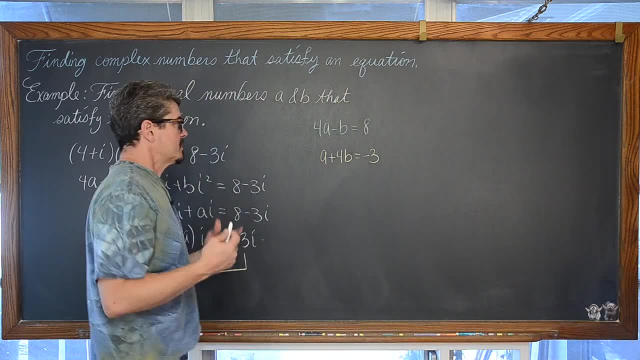 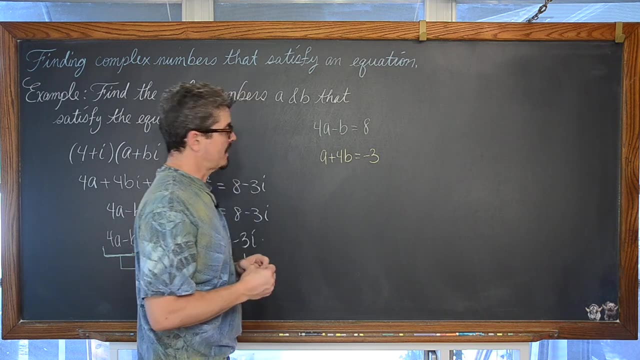 this equation. We are just going to solve this little system of equations. I am going to do this with linear combination or you can do substitution. It is perfectly set up for that. basically, We have: a is equal to negative three minus four b. I want to multiply. 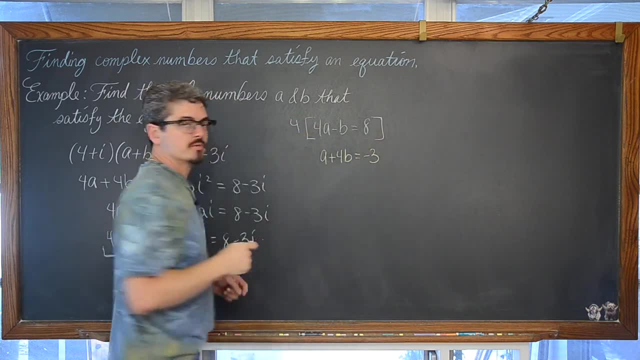 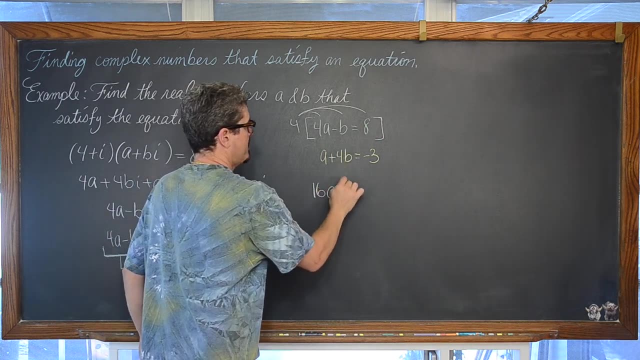 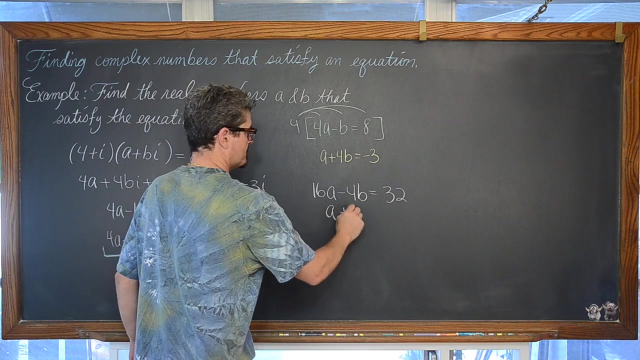 this first equation by four, because I am going to do linear combination. We have four. nope, we have 16a minus 4b is equal to 32.. We have a second equation, of course, of 1a plus 4b. 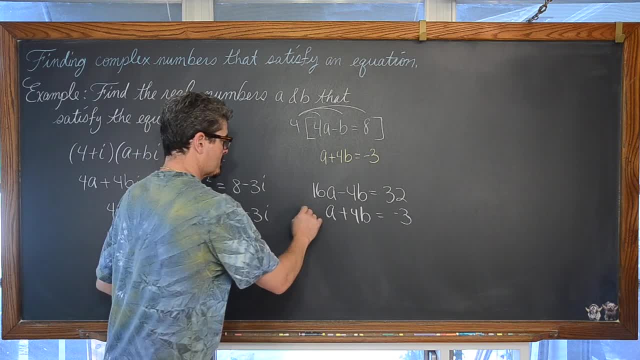 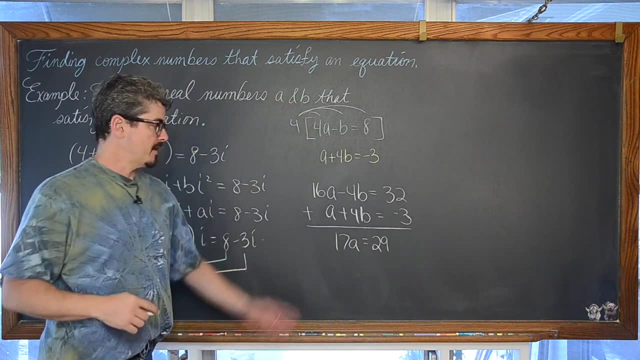 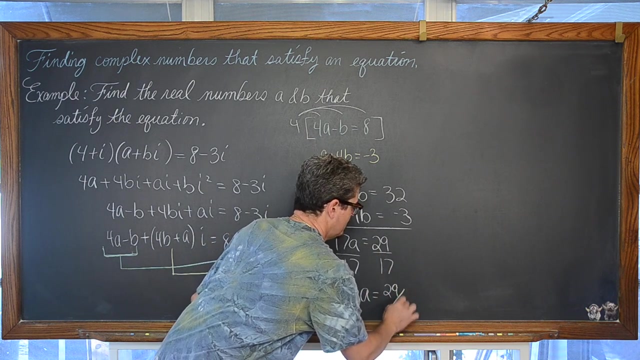 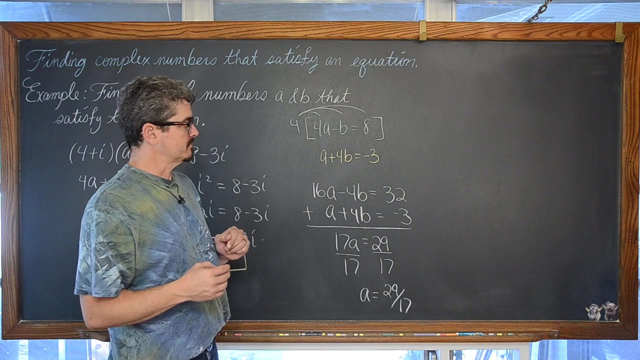 is equal to negative three. We have our opposite coefficients here. We are going to add these equations. We get 17a is equal to 29 and divide both sides by 17, and we have a is equal to 29 over 17.. Well, now that we know what the value of a is, we can plug it into either one of these. 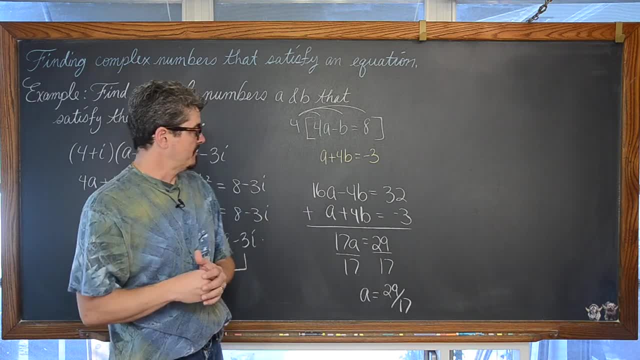 linear relationships, comparing a and b together and solve for b. So we have, let's say that we have here a, which we now know is 29.. We can plug it into a and b and solve for b. So we have, let's say that we have here a, which we now know is 29.. We can plug it into. 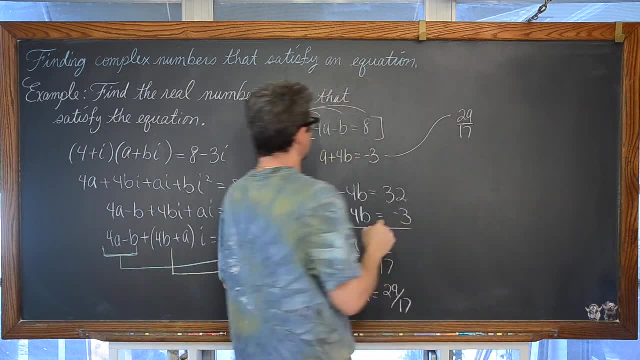 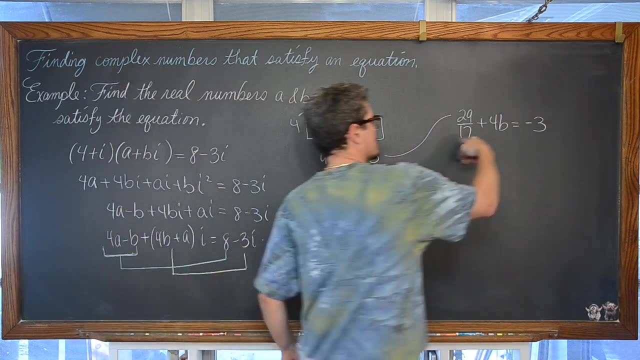 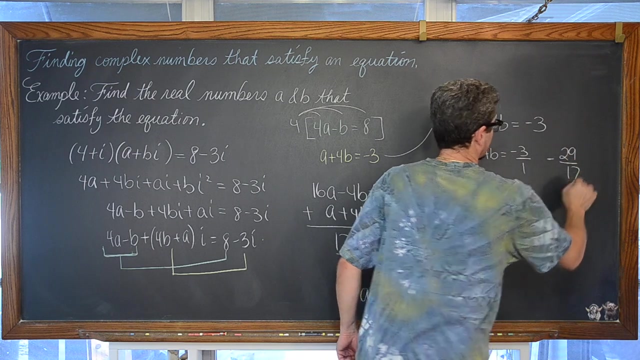 29 over 17 plus 4b is equal to negative three. We are going to subtract both sides by 29 over 17.. As you will see, a little bit of an issue here as I make up my own problems to make these videos Going to get a little bit nasty. here We are going to multiply this. 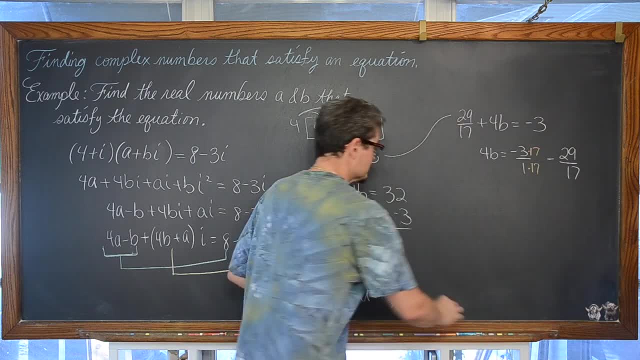 by 17.. At least in the sense of trying to do this in my head. To do so we have: 4b is equal to negative three and b is equal to 17. We multiply both sides and we are getting a degree of alternative here on the same amount of quieres going on. So there is an negative. 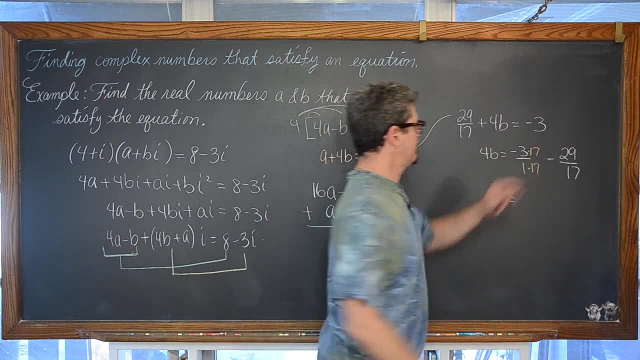 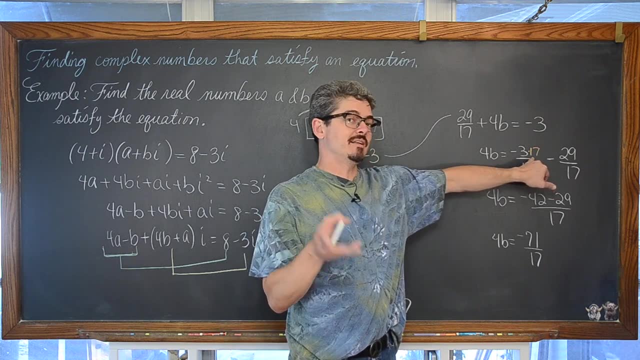 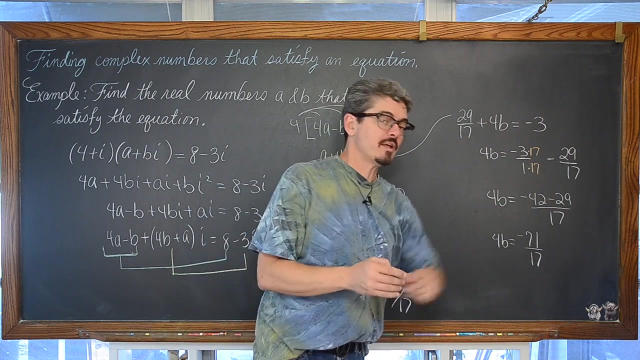 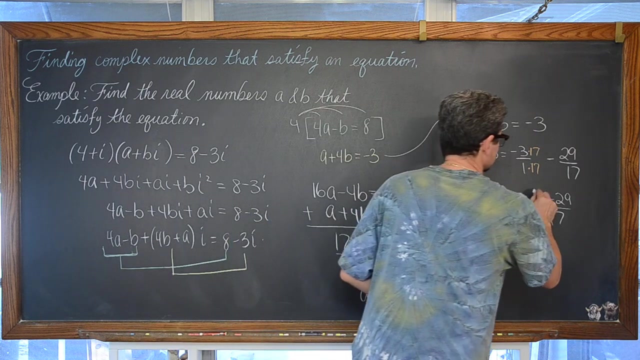 is equal to negative 42.. Yes, Should have just spoke this out as I was doing the problem. Three times ten is thirty, and three times seven is twenty-one, and thirty and twenty-one do not make forty-two, it makes negative fifty-one. So negative fifty-one minus twenty-nine is 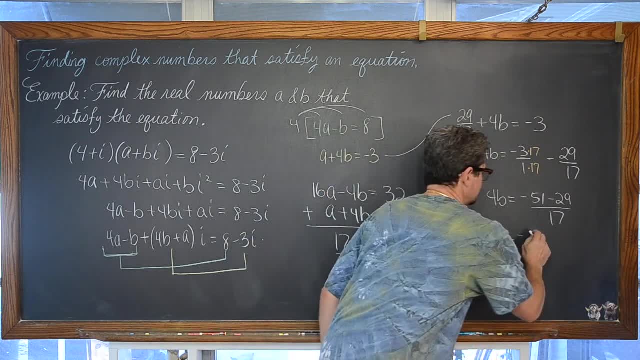 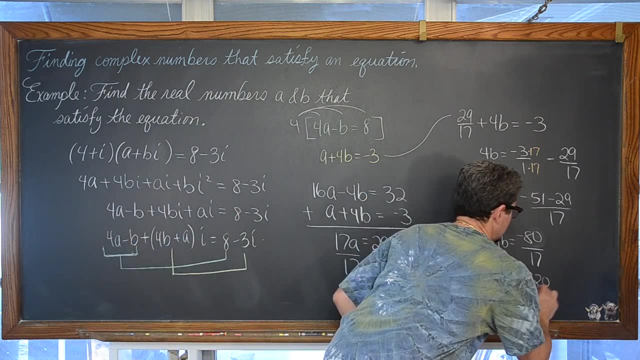 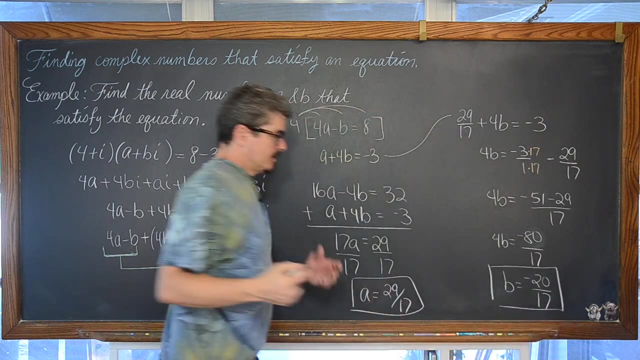 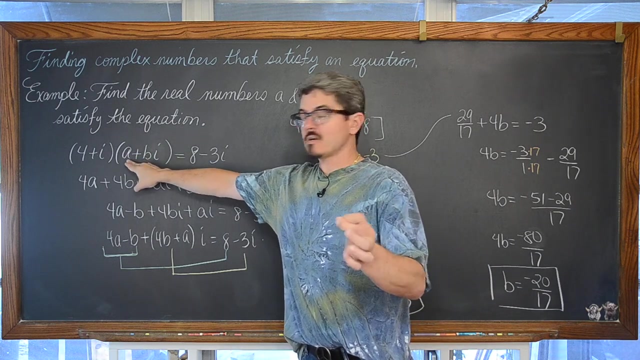 going to give us negative eighty. Divide both sides by four and we get that b is equal to negative twenty over seventeen. So that is one way of solving for the real values of a and b, basically our real portion of this complex number, the unknown complex number. 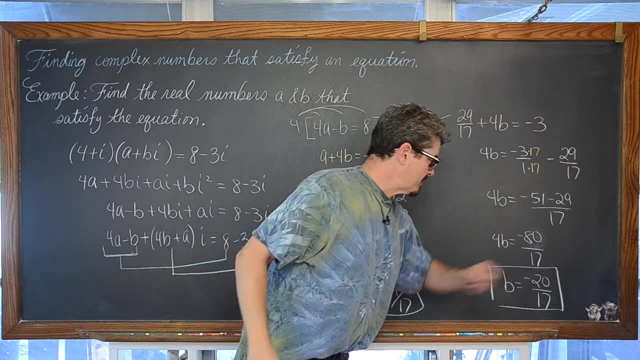 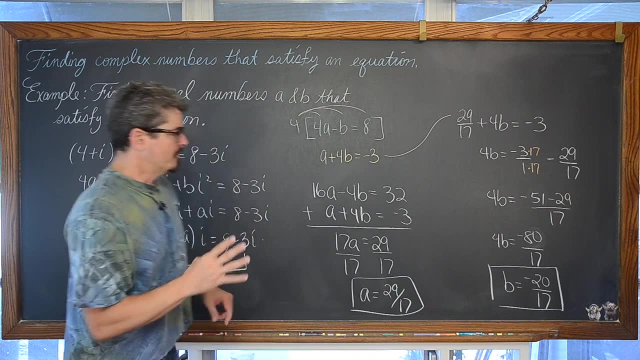 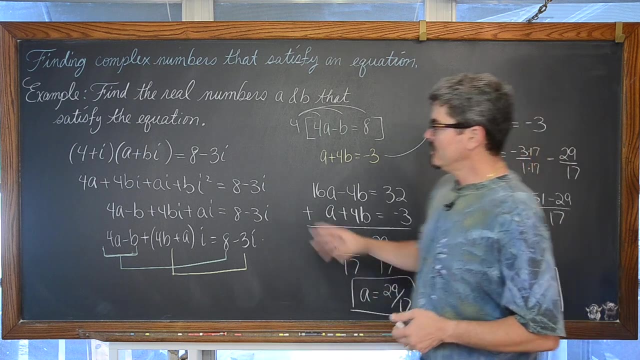 in our original equation, and b, which is the, So b takes on the value of negative. twenty over seventeen. Double check, Perfect. Now you are going to see plenty of problems, I am sure, in your textbook and class, where 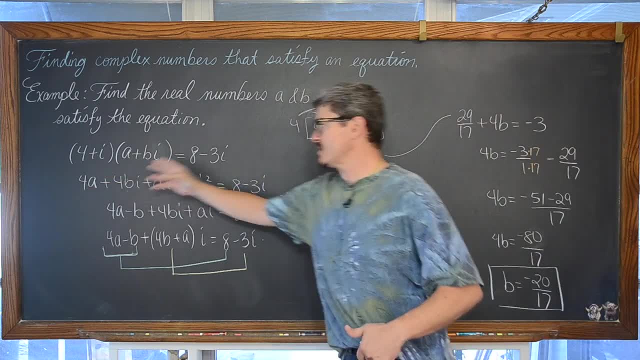 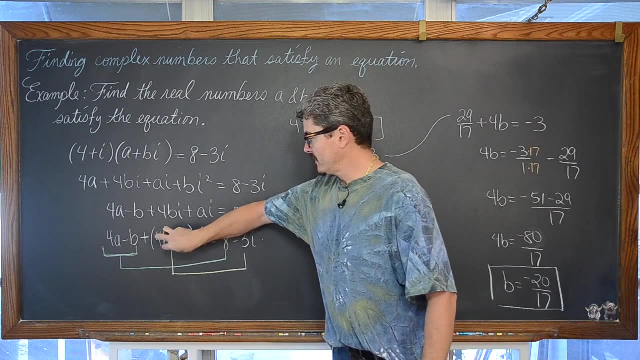 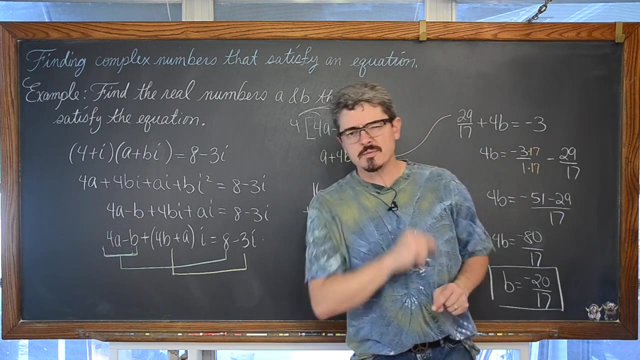 you have just terms all over the place on each side of an equation and you want to compare the real terms and set up an equation from that with the coefficients of your imaginary terms, and create a system of equations. This particular question could have been solved a lot quicker. That example or version. 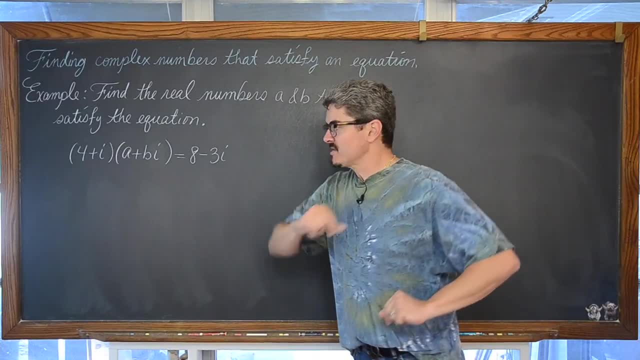 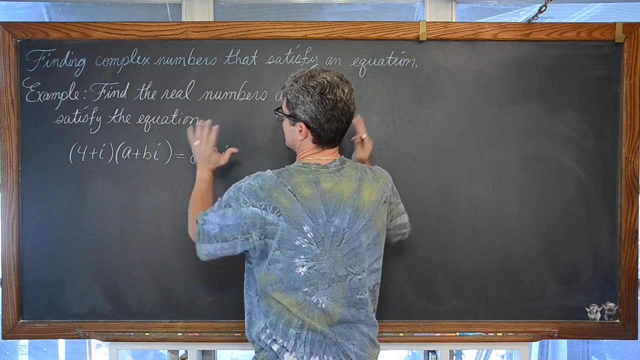 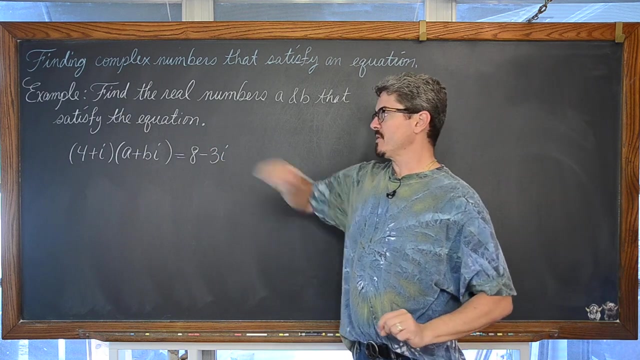 is coming up right now And with our board reset, going back to our original problem, you might do the second technique, had I actually asked for the complex number that satisfies this equation and had a z here, But nonetheless, instead of distributing the four plus i with 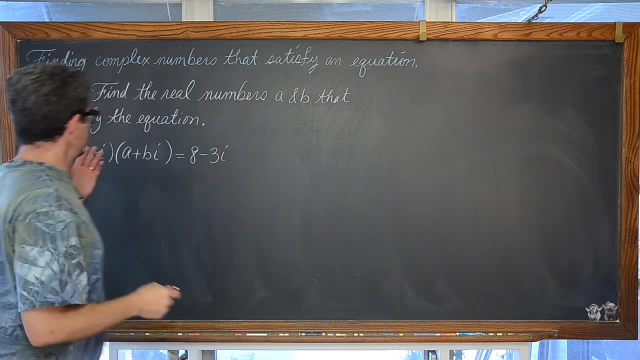 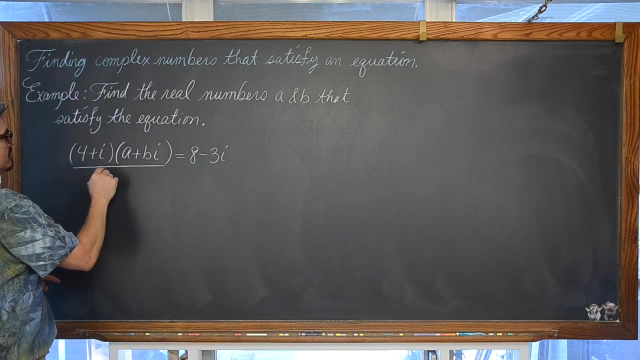 the a plus b i. you can just You know. if this is the variable you are looking for and it is multiplied by a two, you can just substitute the two by a two and you will a known quantity. you can just divide that away. You might have been watching me do that. 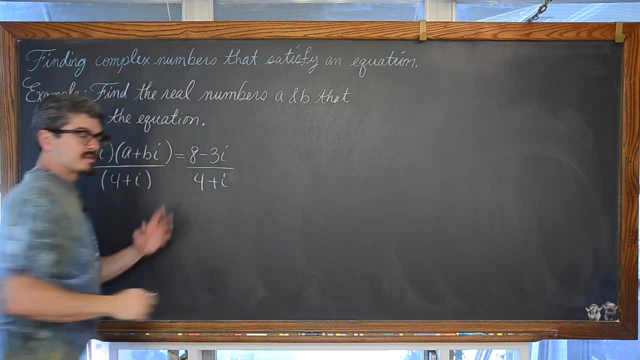 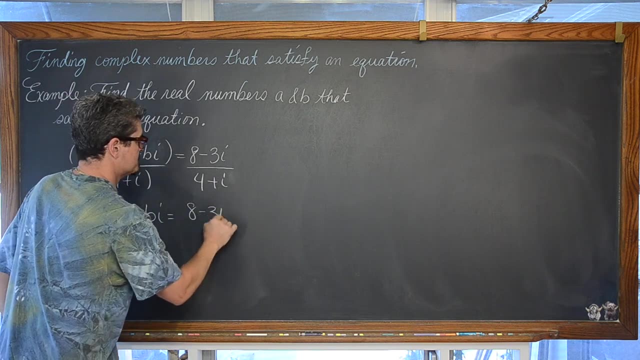 example, and just wondering why I didn't do this in the first place, Because the techniques in that previous example may come in handy And we don't always do questions the most efficient way when we are first learning a concept or even when we are super comfortable. 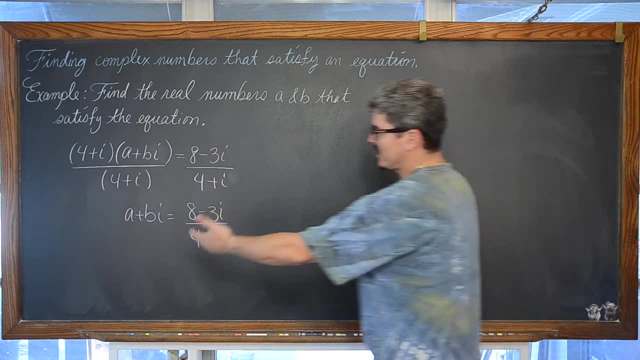 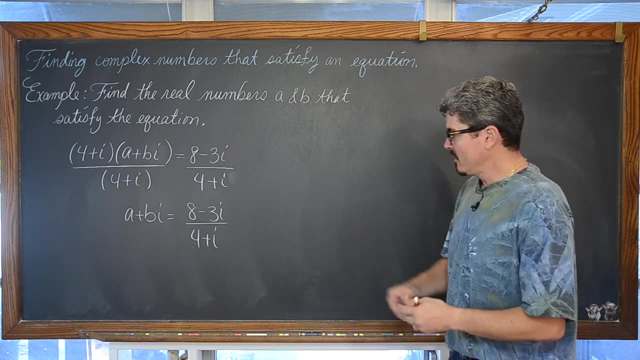 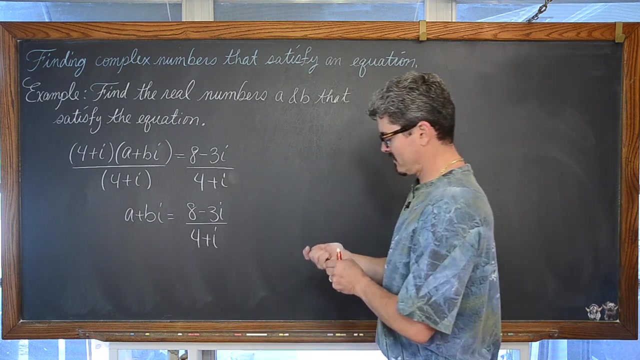 with what we are doing. Yeah, this complex number a plus bi is just a quotient of two imaginary or two complex numbers. We don't like to leave i in the denominator of a fraction, kind of like leaving a radical in the denominator Usually. we want to rationalize that denominator. 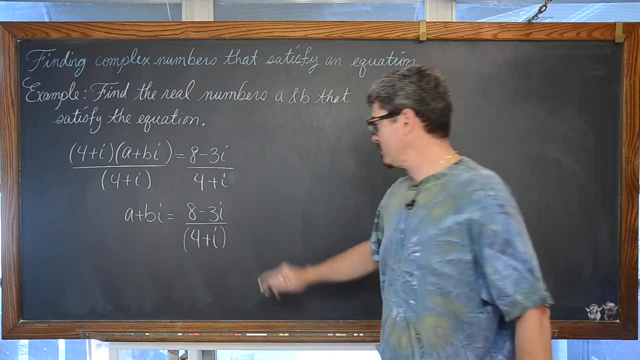 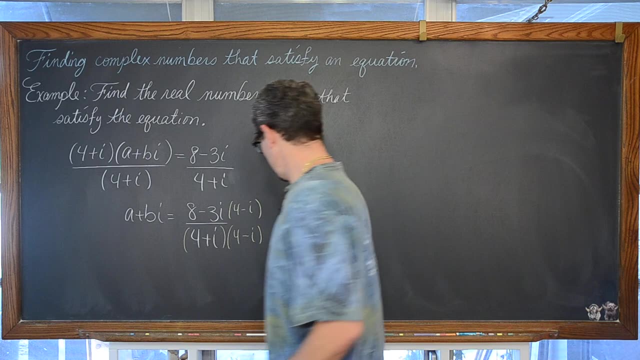 and clean it up. We are going to get rid of this i in the denominator, of course, by multiplying the numerator and denominator by the conjugate And wrap that up. So we are going to get rid of this up in parenthesis and let's go ahead and distribute. We have eight times four. 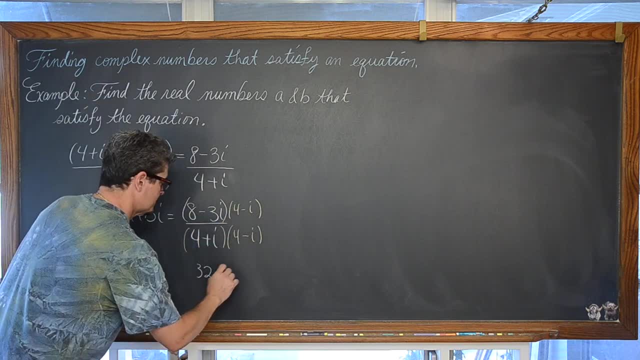 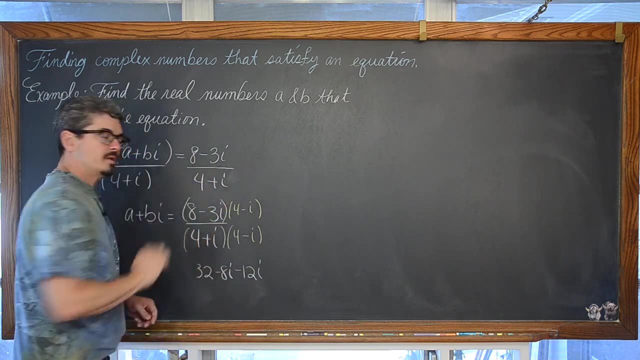 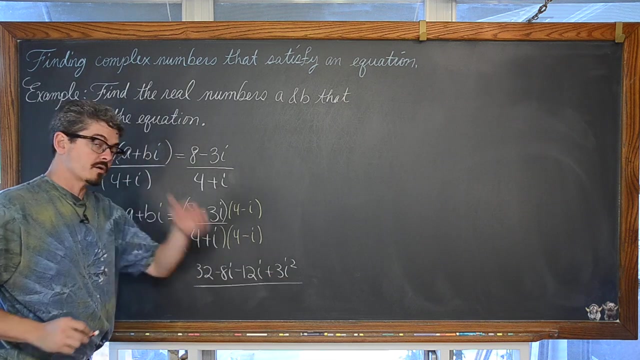 is thirty-two. We have eight times negative i is negative, eight i. Now we are looking at negative twelve i And negative three times four And negative three i times negative i is going to be positive three. i squared, Which we know i squared is negative one And 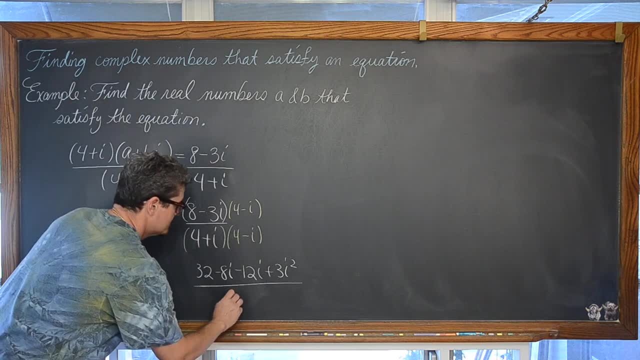 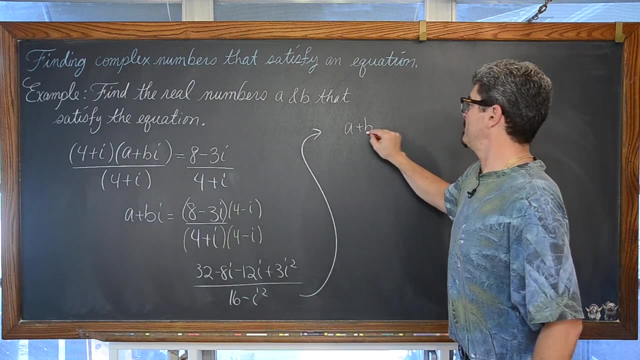 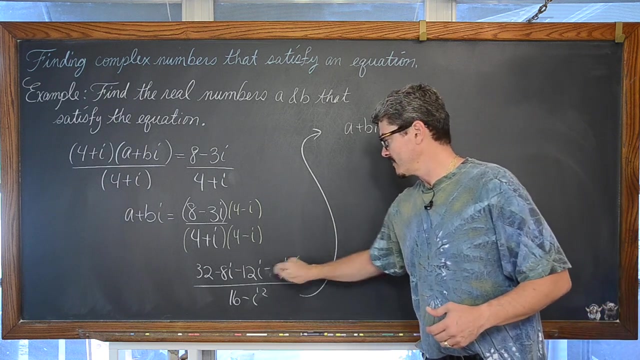 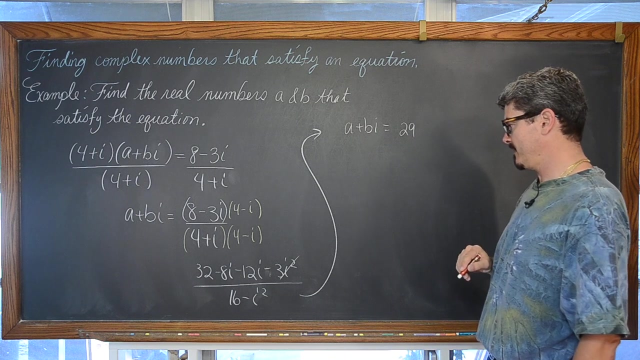 down here we have a difference of squares. This is just going to be sixteen minus i squared. Cleaning that up, we have a plus. bi is equal to now. this is plus three i squared, but really it is minus three. So we have thirty-two minus three, which is going to give us that twenty-nine. 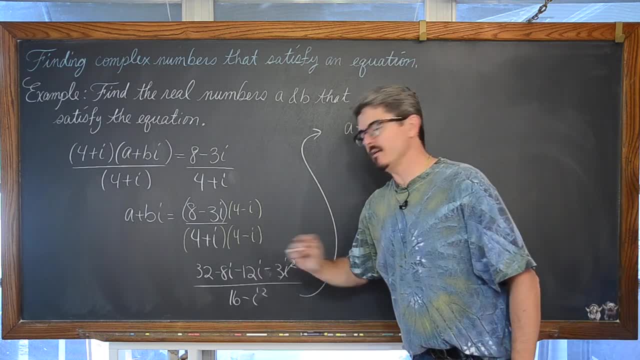 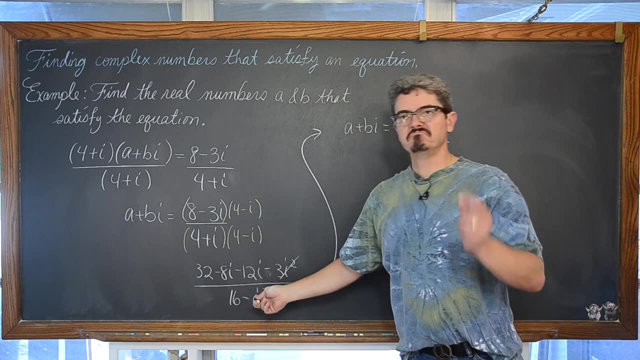 that we had before, And we also have negative eight i minus twelve i, which is negative twenty i over sixteen minus negative one. So that's going to give us twenty-two minus three And that's going to give us sixteen plus one. Sixteen plus one is seventeen. We want to. 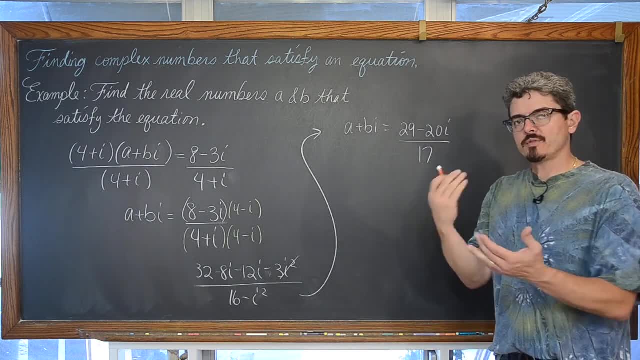 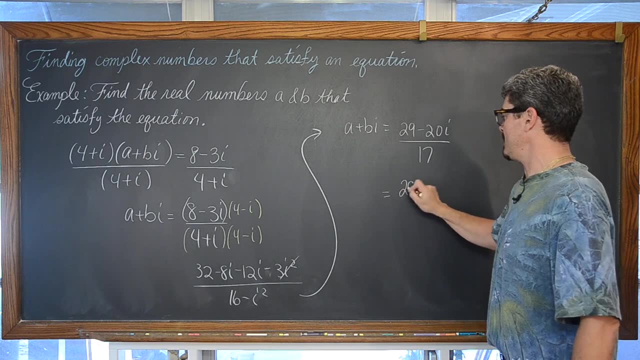 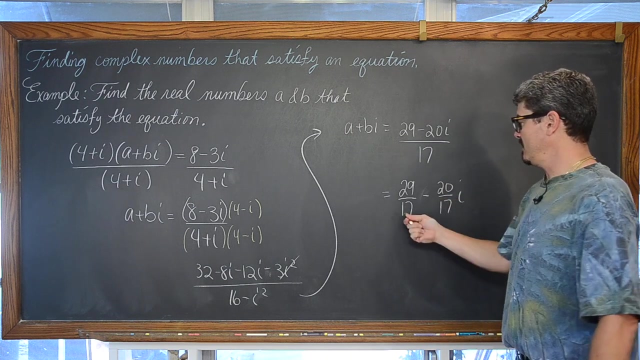 write our complex numbers with a real and an imaginary part, So this is not sort of appropriate to write this. We have: a plus bi is equal to twenty-nine over seventeen minus twenty over seventeen. i. And here is your value of a And here is your value of. 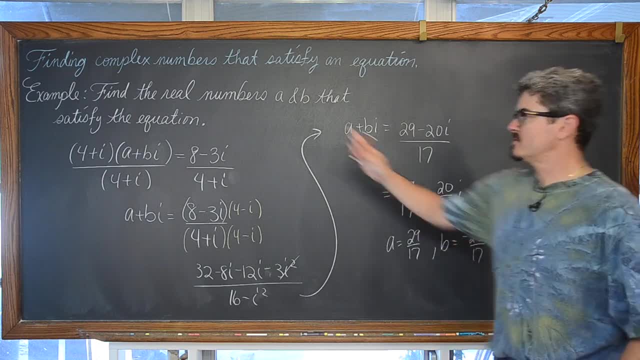 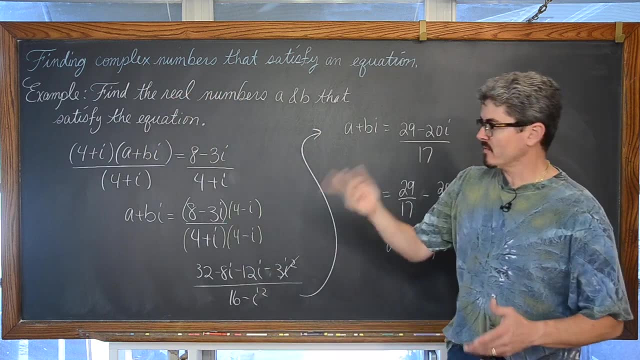 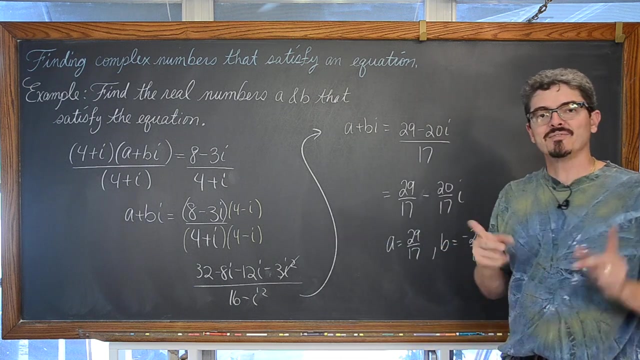 b. So we had two ways of solving or finding the complex number or the coefficients within that complex number, the real and imaginary coefficients that satisfy this equation. And yeah, one technique was a lot quicker than the other, but here we got the same answer. 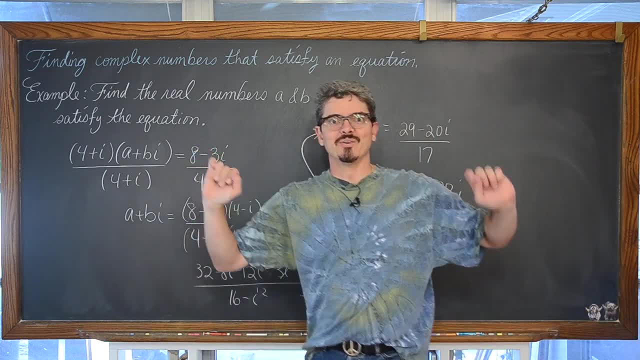 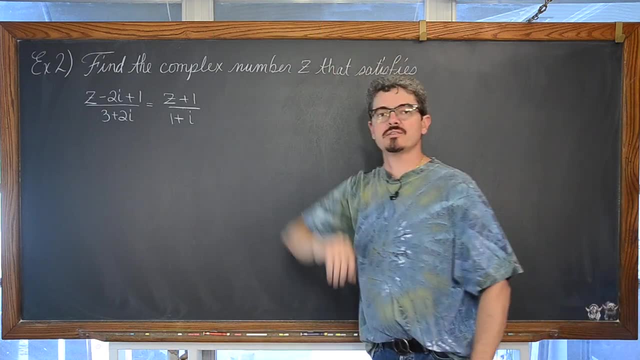 And really that's all that matters. Our second example coming up right now. Alrighty, then our second example. We are going to find the complex number z that satisfies this equation Where we have z minus two, i plus one. And we are going to find the complex number z that satisfies this equation Where we have z minus two, i plus. 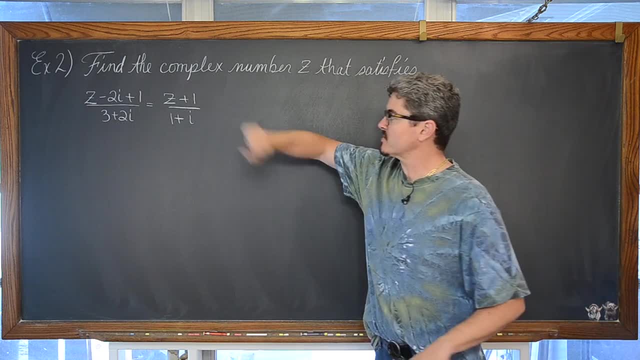 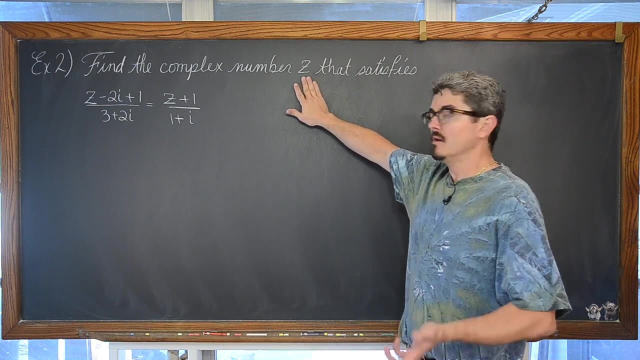 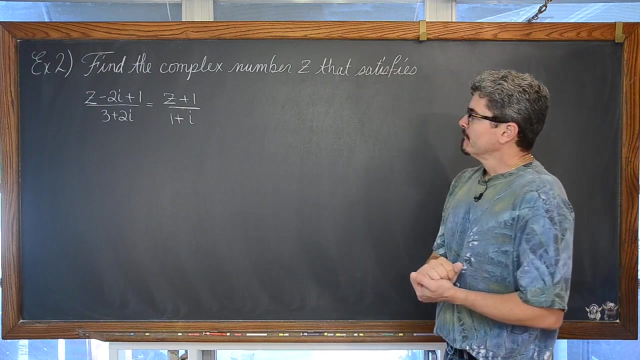 one over three plus two i is equal to z plus one over one plus i, And so I am telling you here that everywhere in the equation that you see, a z we are looking at. you know, that is our complex number, That is our a plus bi. Okay, Well, we have an equation where 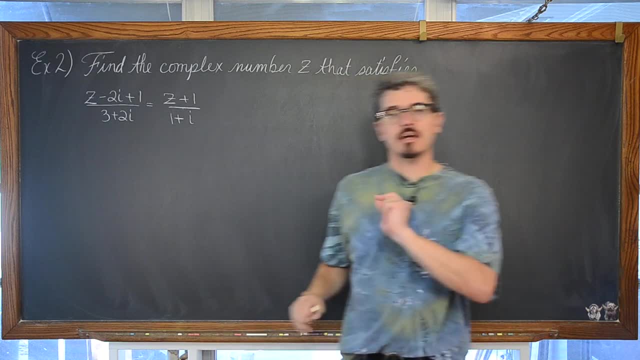 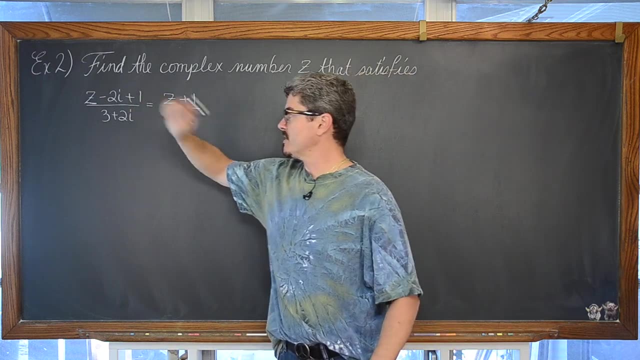 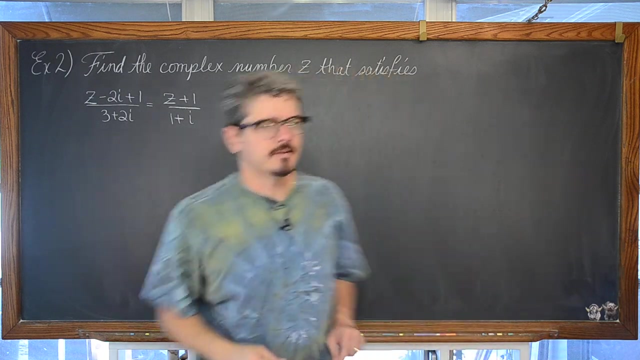 there is one fraction on each side. And how do you go about this? You basically multiply both sides of the equation by Three plus two. i times i plus, excuse me, one plus i, or you cross multiply. So we are going to go ahead and cross multiply this and we are going to get z minus two i We 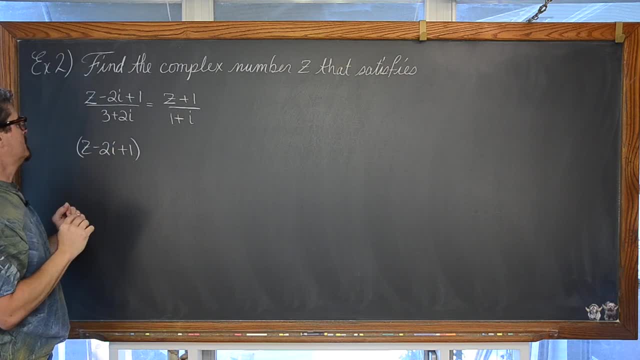 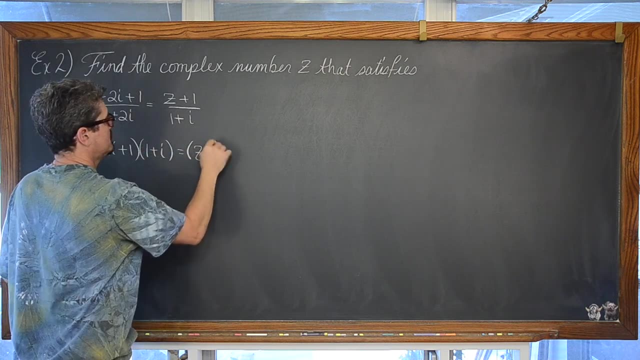 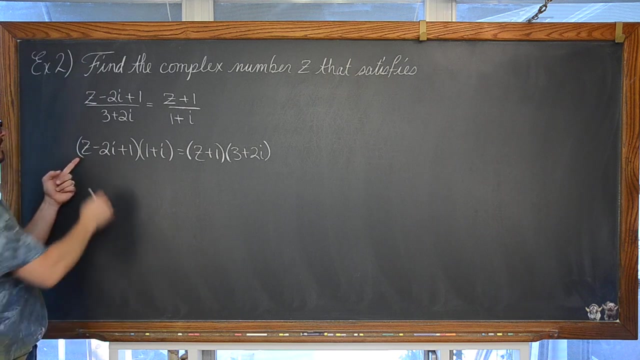 are not really getting anything. I am just showing the multiplication: Z minus two i plus one times one plus i is equal to z plus one times three plus two i plus one. Okay, One I plus one plus z. So that is going toris equal to three times three plus five of i. 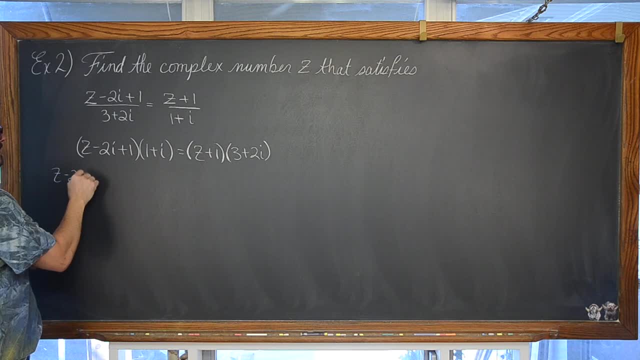 We are going to go ahead a distribute: We have z minus two i plus one times one. So that is just going to be z minus two, i plus one. Now we are going to take the term here of i and multiply it to z minus two, i and the plus one to give us over one, So over. 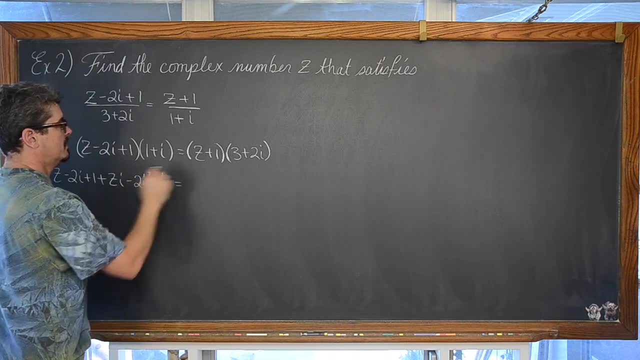 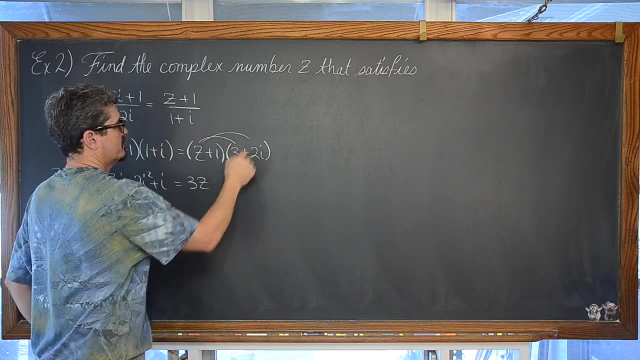 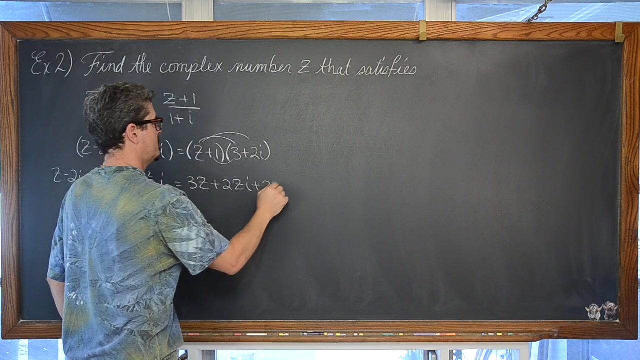 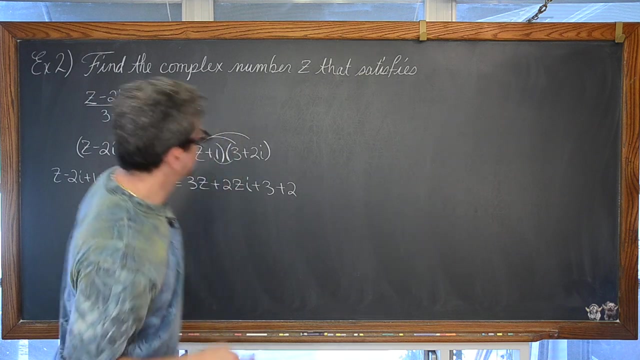 one by 2i squared. �� and we're going to multiply, distribute together these two binomials. We have 3z and then we've got plus 2zi. Now we've got plus 3 plus 2. That is supposed to be a 1, right? Yeah. Plus 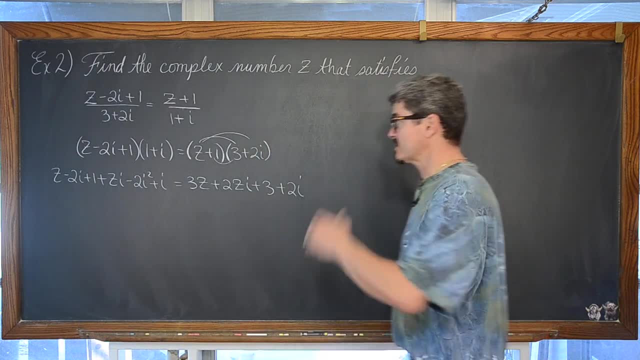 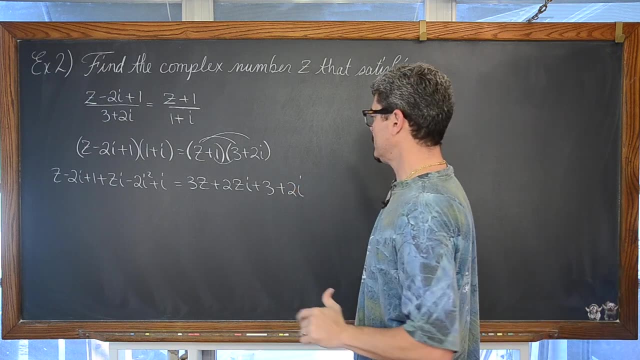 2i. I hate to do this whole example and realize I miscopied my problem. Ok, so what's going on here? Well, we've got just a tiny bit of cleaning up we can do. It seems like we have a big old mess here. We have i squared, which is negative 1.. So this is going to become: 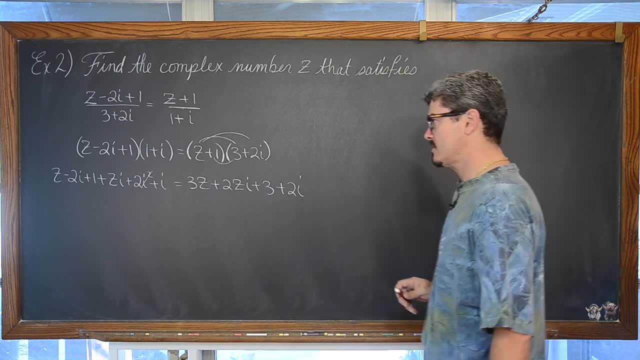 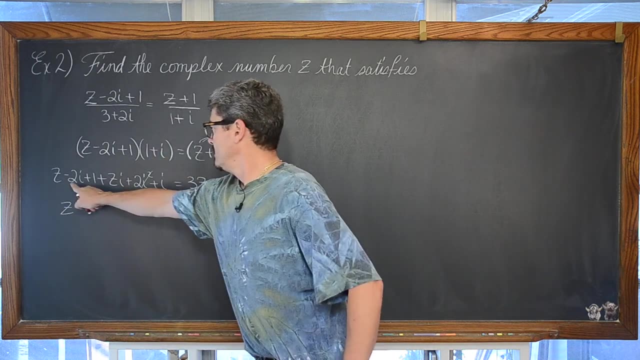 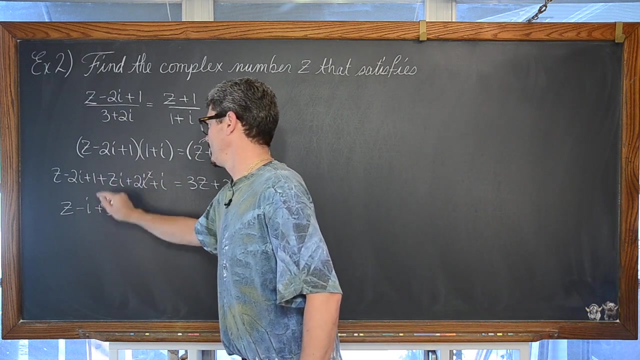 just plus 2.. And we've got some like terms here. So we're looking at z Negative 2i plus i is negative. i We've got 1 plus 2, which is 3.. Plus z squared, which is negative 2i. 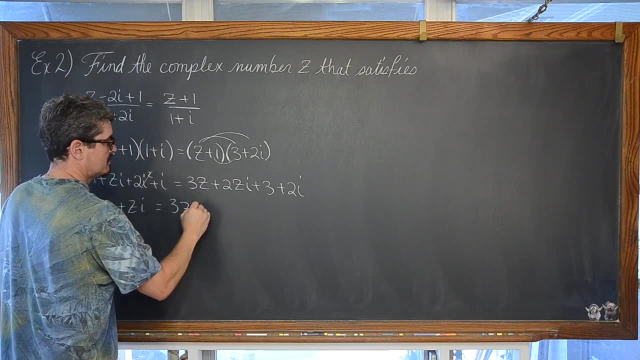 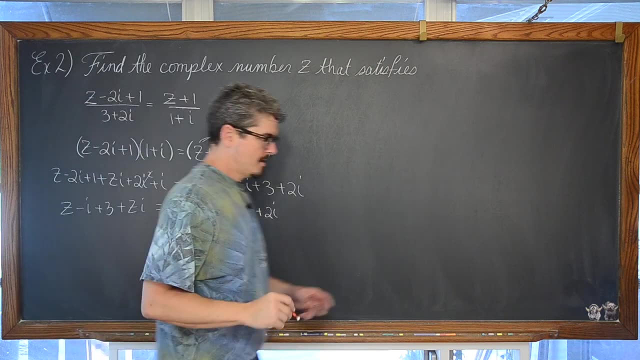 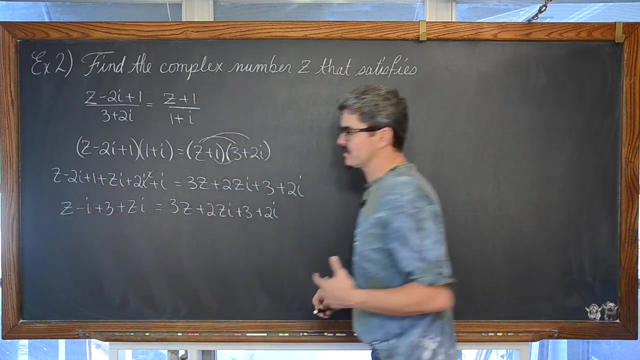 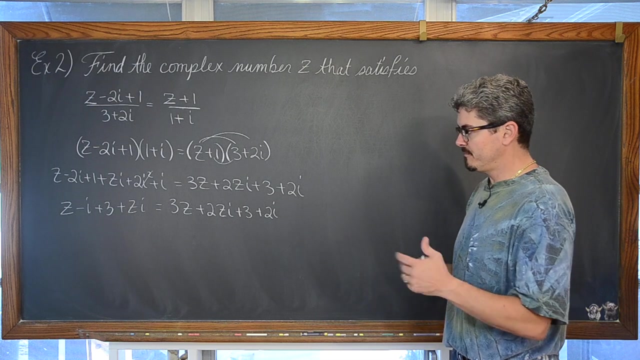 zi is equal to 3z plus 2zi plus 3 plus 2i. Now here's why I kind of did the first example. in two different techniques We've got basically sort of like real terms. Well, we have terms without i's and terms with i's all over this equation And we basically want to compare. 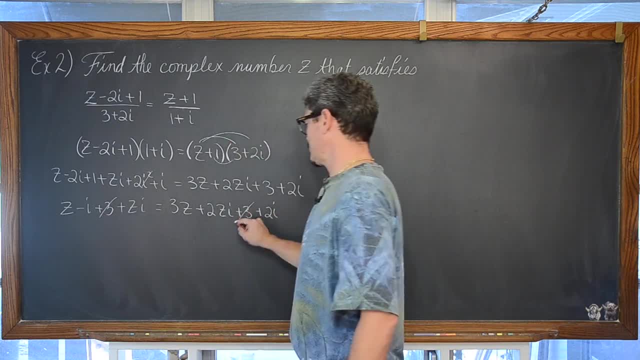 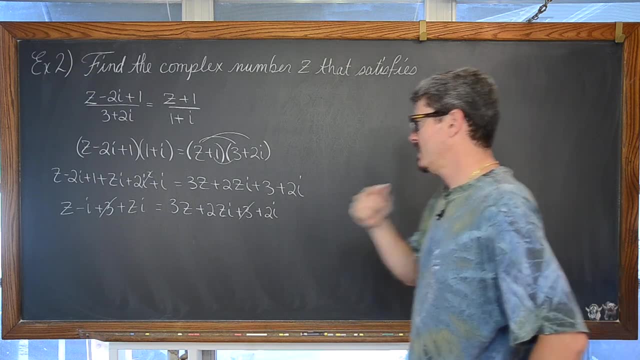 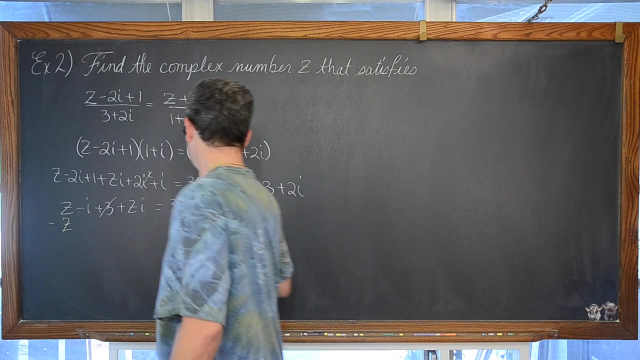 them. So what can we do? We can subtract both sides by 3, which is going to cancel that out, We've got. we can subtract both sides by z. We can. you know, we're trying to solve for that complex number. We're trying to solve. 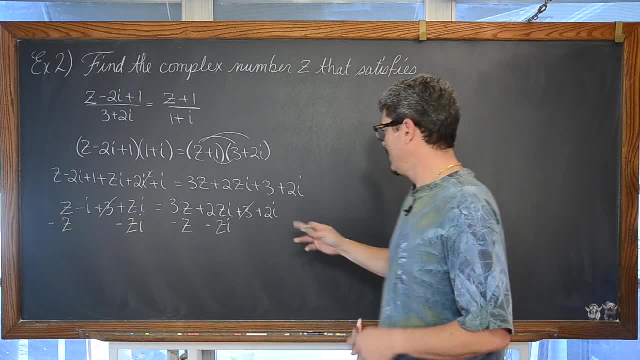 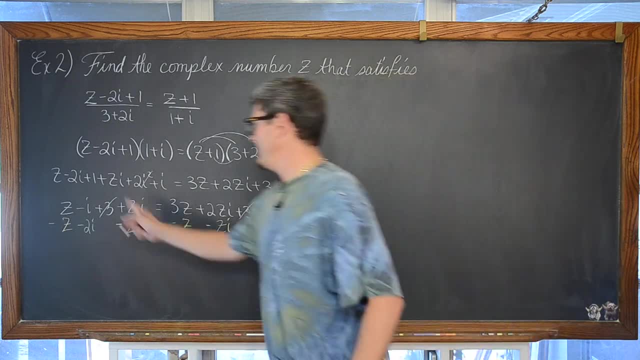 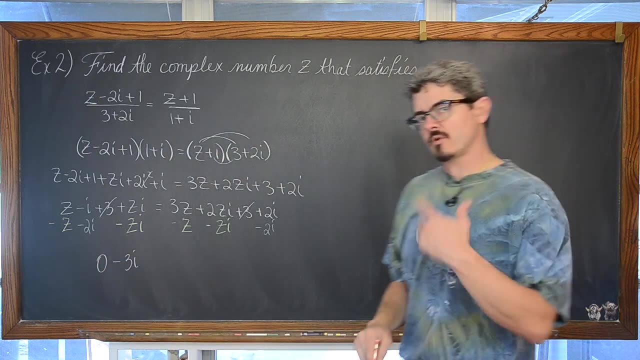 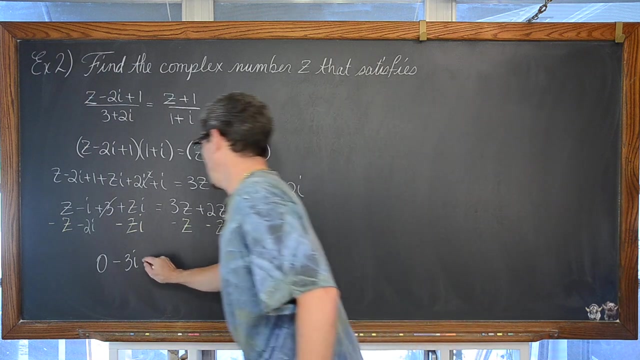 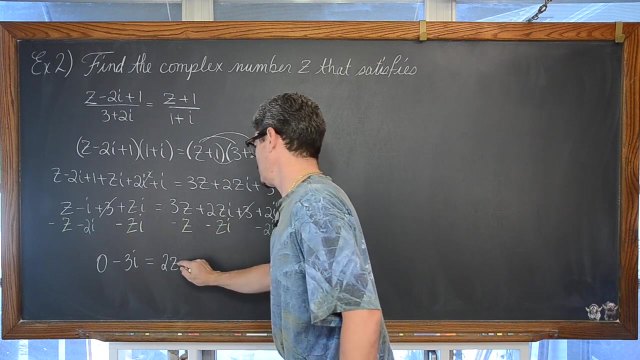 2i, And when we move all these terms around we get negative. 1i minus 2i is negative 3i And, just for good measure maybe, show that there is a zero, a real plus an imaginary portion for this complex number. And we've got 3 minus 1 is 2z And 2 minus 1 is 1.. So 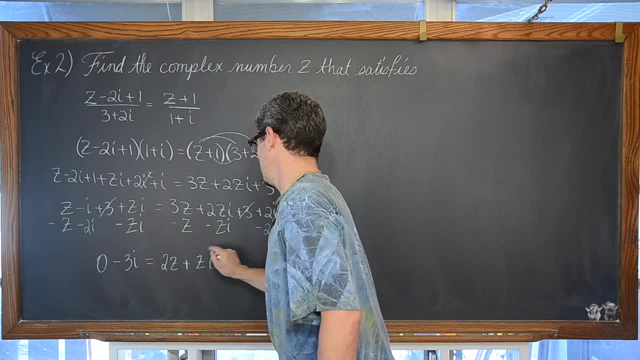 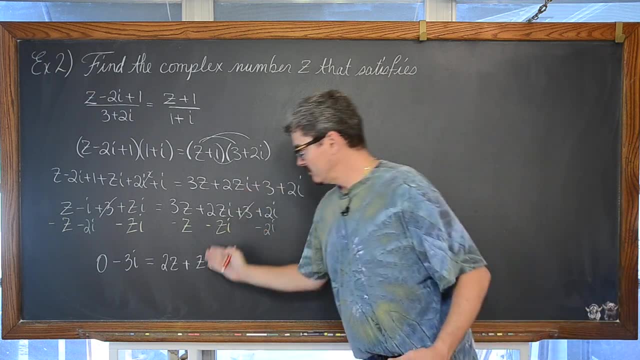 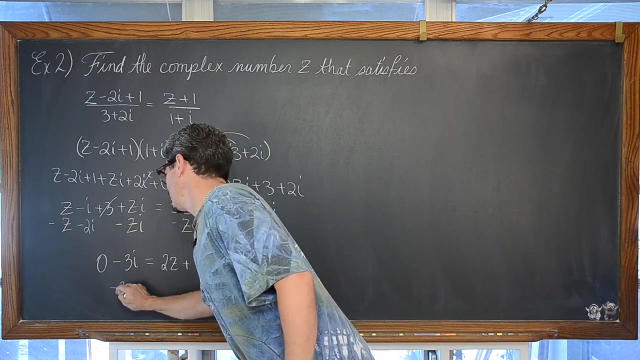 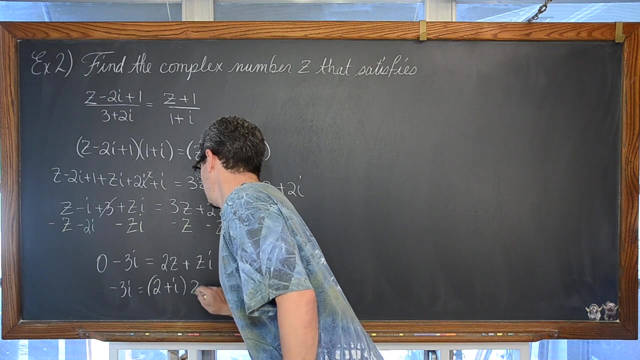 we have plus zi- Excellent. Now keep in mind that we're trying to solve for z. We need to rewrite this right hand side, Do a little factoring so that we only have z showing up once. So we're going to factor out a z And we have negative. 3i is equal to 2 plus i times z And we're starting. 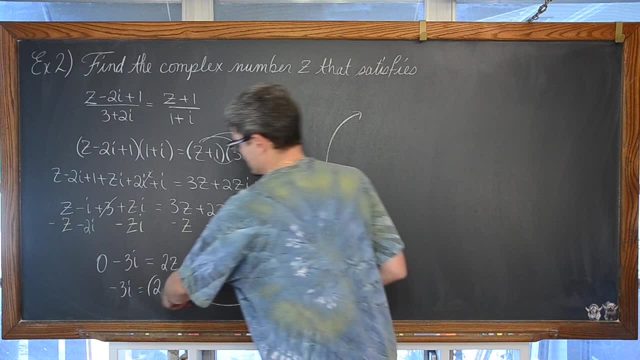 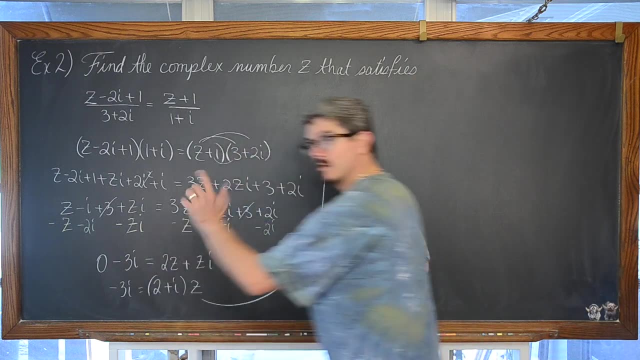 to see the end of this come out very, very clearly now. We're going to divide both sides by 2 plus i And get, And I'm going to put the I'm going to. This is going to be an equal sign, so I'm going to swap sides so I have some room to work over here. We. 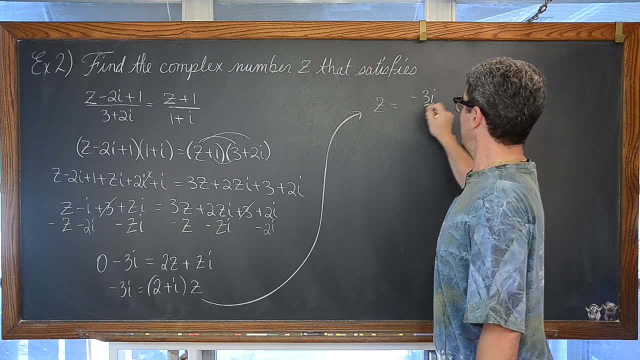 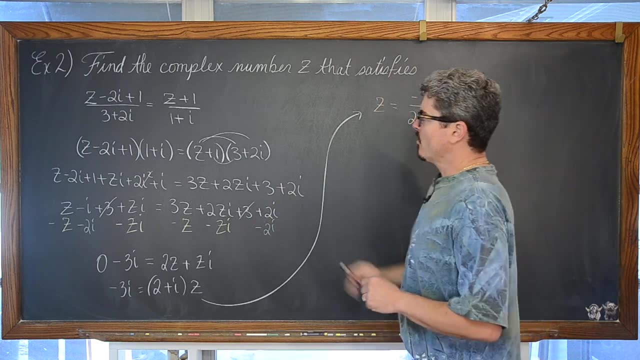 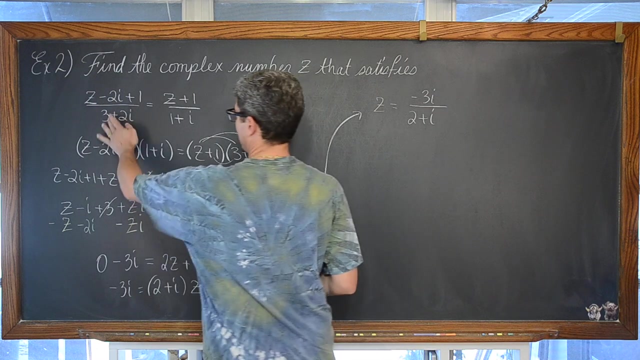 have z is equal to negative 3i over 2 plus i. So we had a new style of equation. We're asked to basically just solve for z. We're not losing our head, We're kind of pulling on our algebra skills and we have one fraction equal to one fraction. 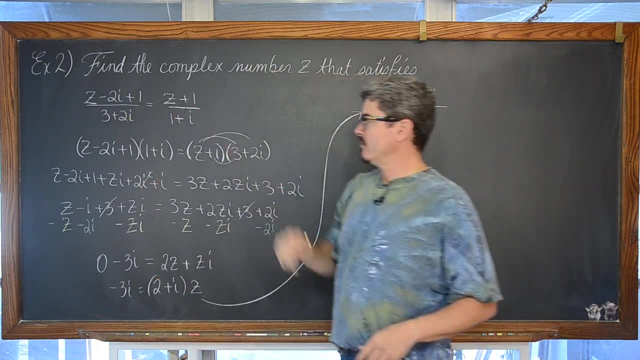 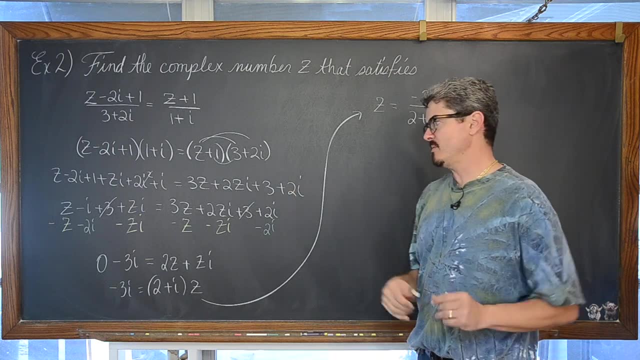 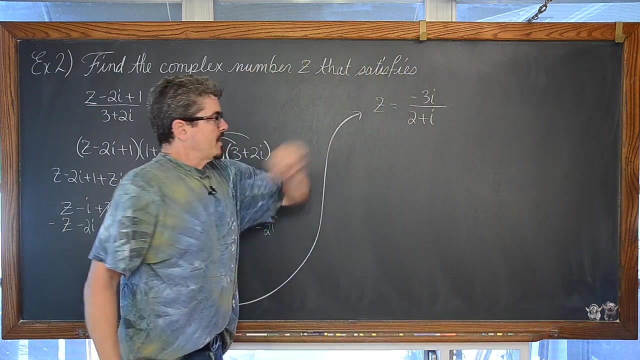 So we're either multiplying by all these factors in the denominator to make the divisions cancel away cross multiplication. It starts to blow up here and look really nasty. but just remember, you are trying to solve for z. Just get that variable together on the same side. Now we 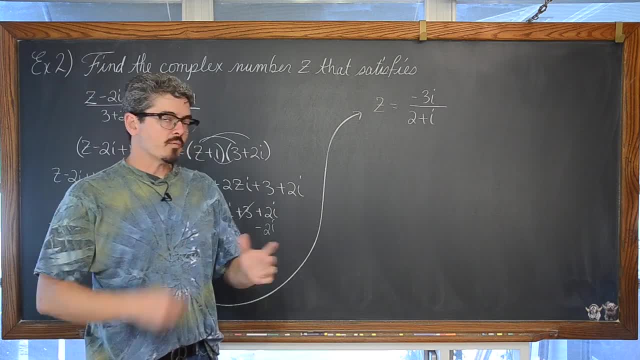 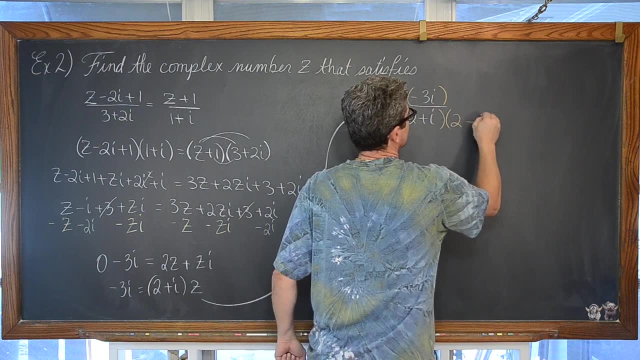 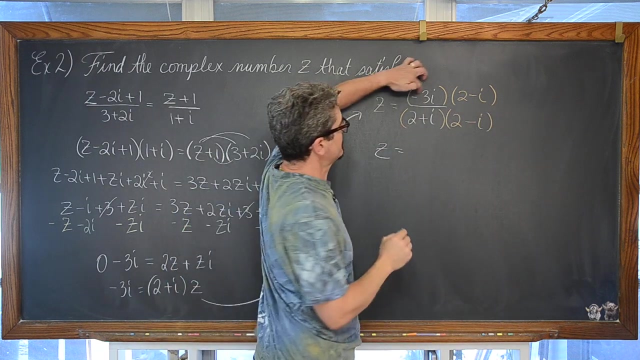 have z is equal to negative 3i over 2 plus i. We are going to clean this up one more time bywell, we have more examples coming, but we are going to multiply the numerator and denominator by the conjugate. We have: z is equal to negative. 3i times 2 is negative. 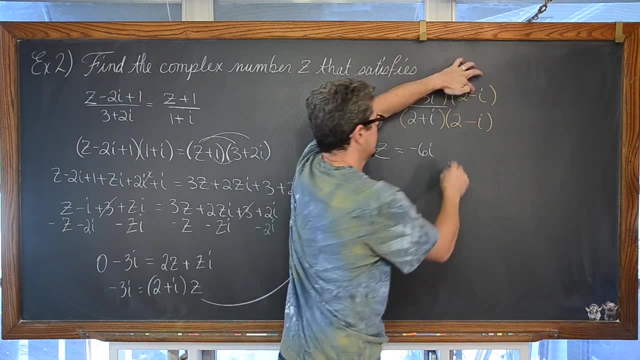 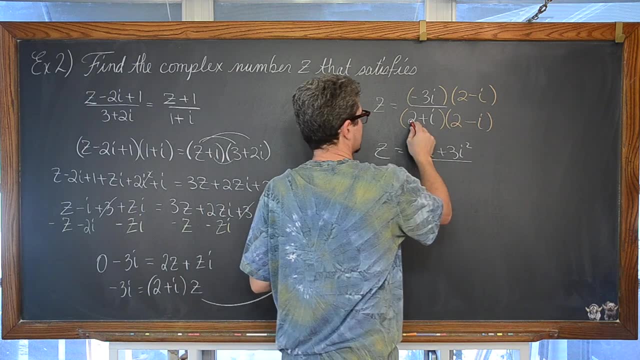 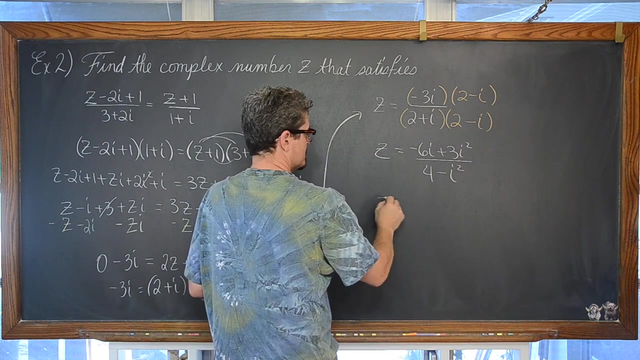 6i And then we have negative times. negative is positive. so we have a plus 3i squared overand this is a multiplication of a difference of squares, basically patterna plus b times a minus b. So we are looking at 4 minus i squared. That means that z is now going to. 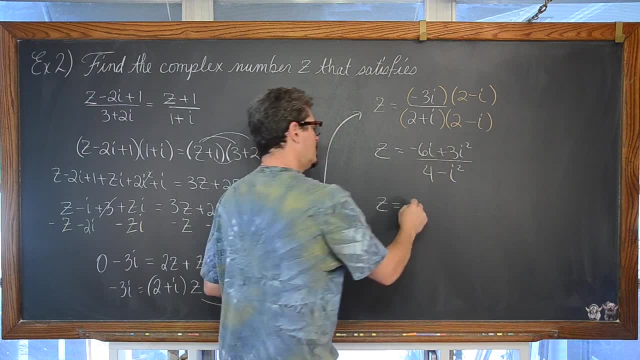 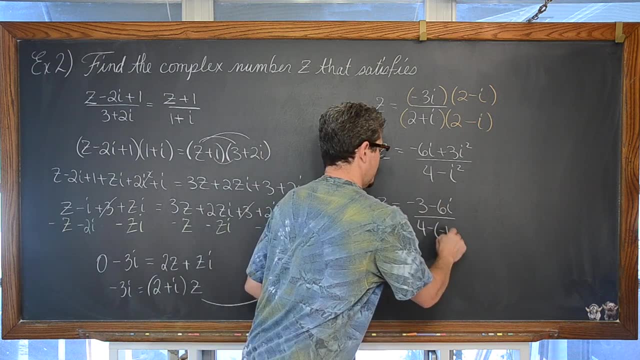 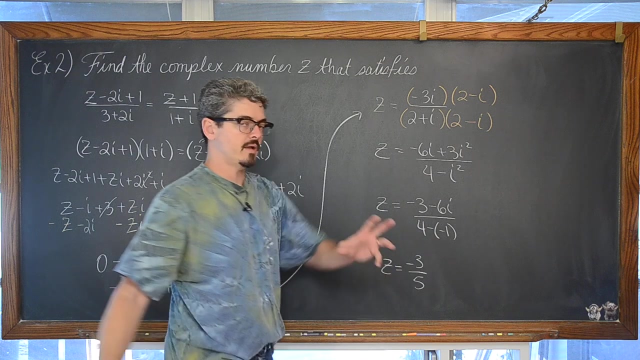 bewith i squared, being negative 1.negative 3 minus 6i over 4 minus negative 1.. So we haveand that is going to give us a final answer of negative 3 over 5.. You want to write? 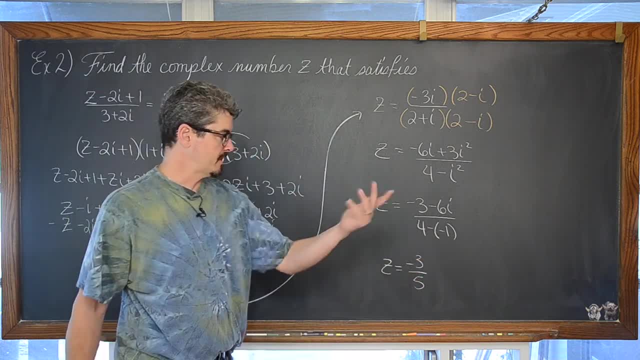 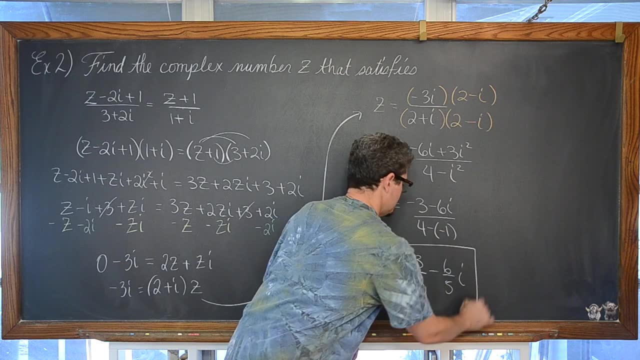 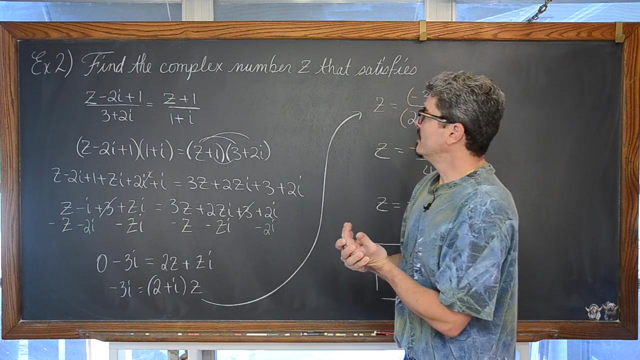 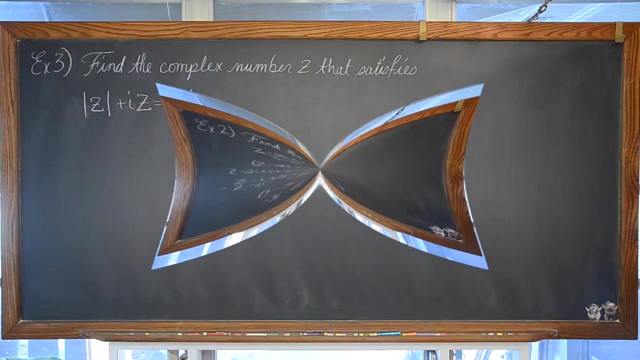 your complex number with a real portion or term and an imaginary termminus 6 over 5i, And that is the complex value number that satisfies this equation. Example 3 coming up right now. Third example: A little bit of a twist with each one of these new problems we have got. 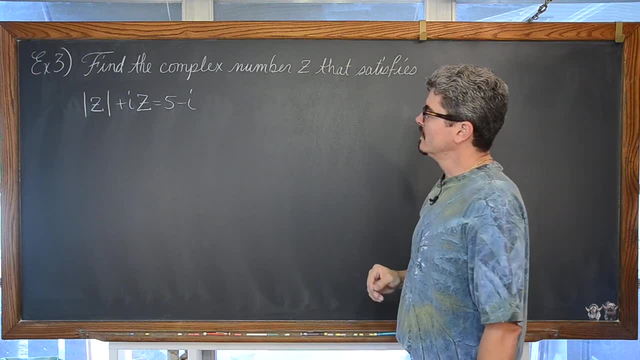 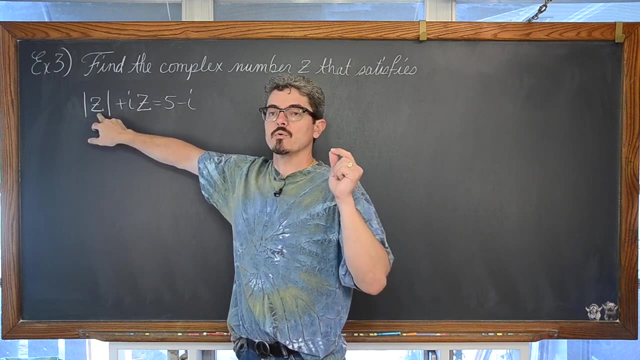 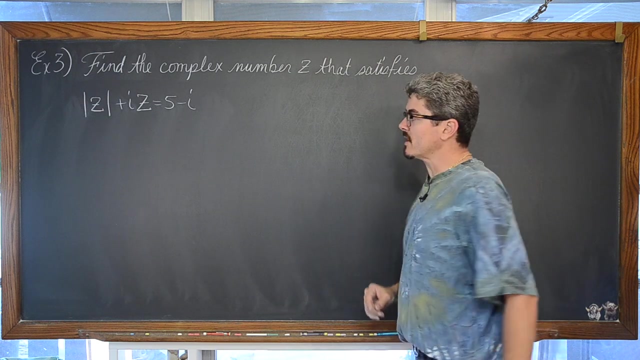 Find the complex number z that satisfies this equation. Ok, Remember this absolute value. looking function around our complex number is asking for the modulus of this complex number, And that is going to help usyou knowdirect us into the direction that we. 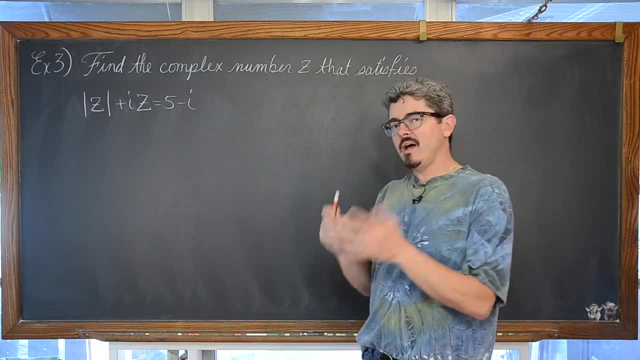 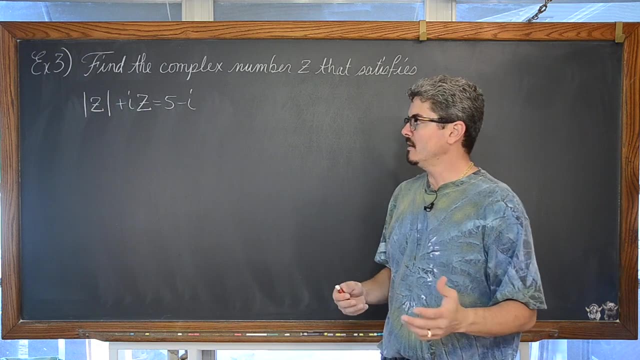 do this problem, or how we do this problem Now, becausewe are going to do this problem, we have got this modulus notation in this equation. It is not something that we are going to just be able toyou knowsolve for z. It is kind of hiding the mathematics. 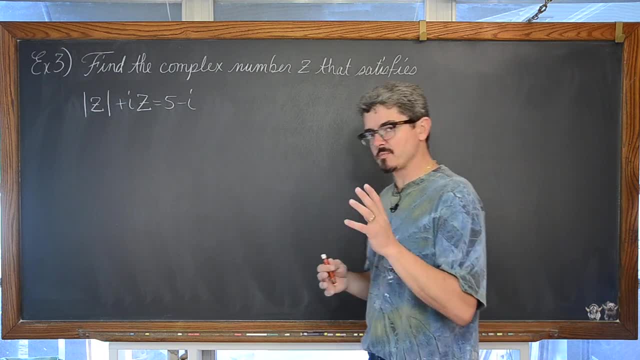 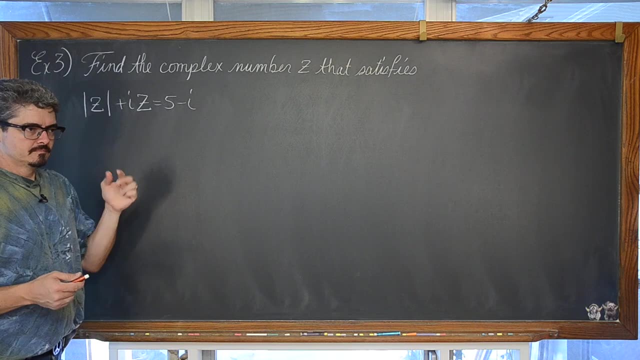 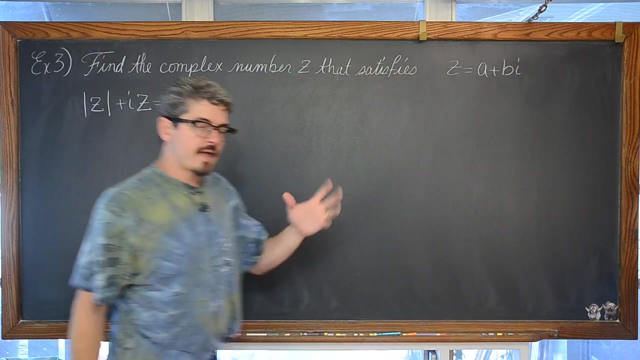 that you need to tackle to do this problem. So, for this particular one, we are going to remember that z is actually representing this complex numbersort of that standard form, if you willof a plus bi. So we are going towe are going towe are going. 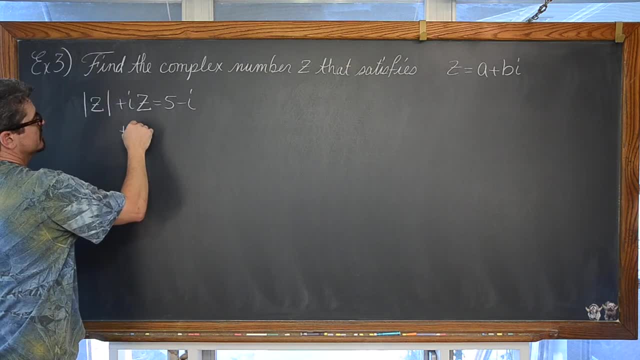 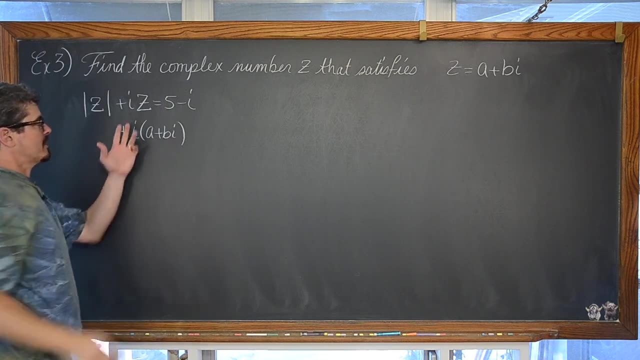 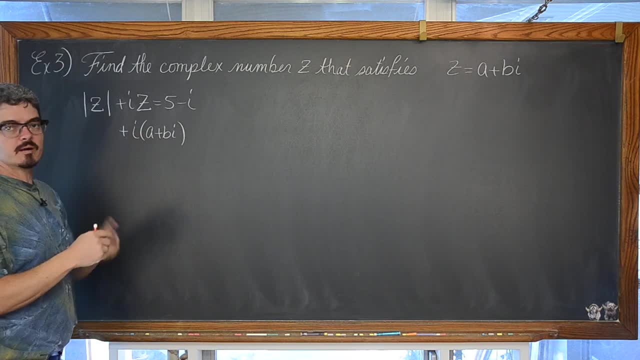 you go. I already have i in here. Nonono, It is i times that complex number is equal to five plus kioopsminus i. Now, by bringing in the fact and using the fact that z is equal to a plus biI am actually writing this outjust to this information that I. 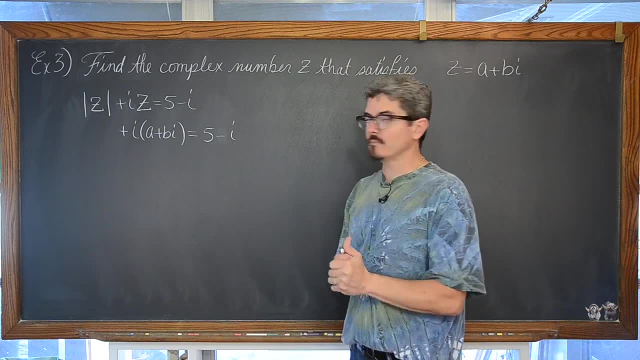 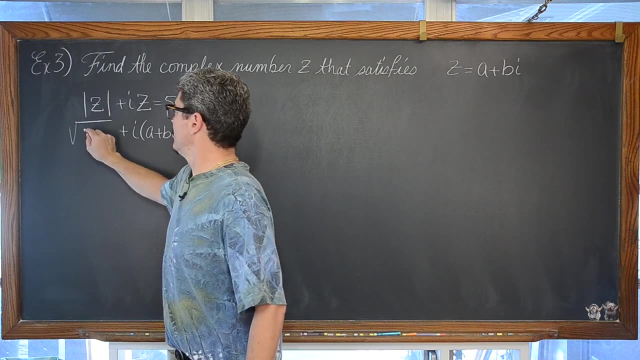 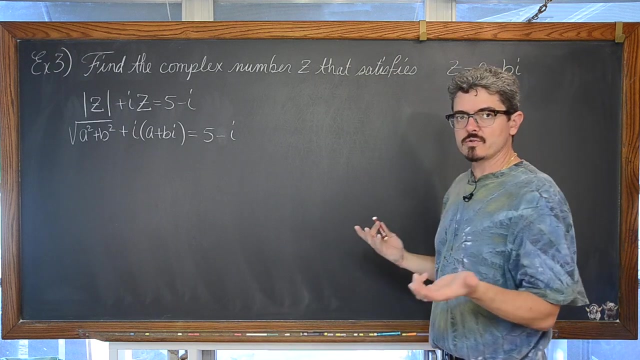 out the two terms of this complex number, then that allows us to recall here that the modulus of z is the square root of a squared plus b squared. Okay, so let's just start doing the algebra. We have an equation with a square root in it. You know, back in Algebra. 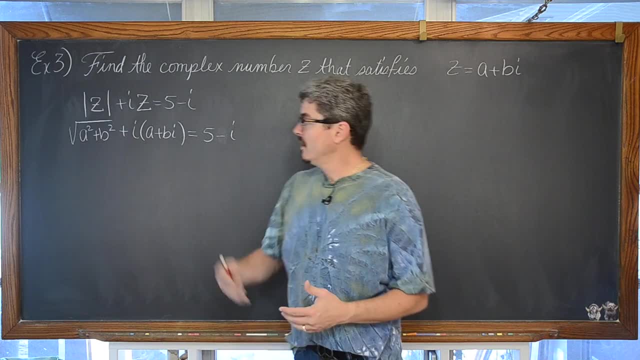 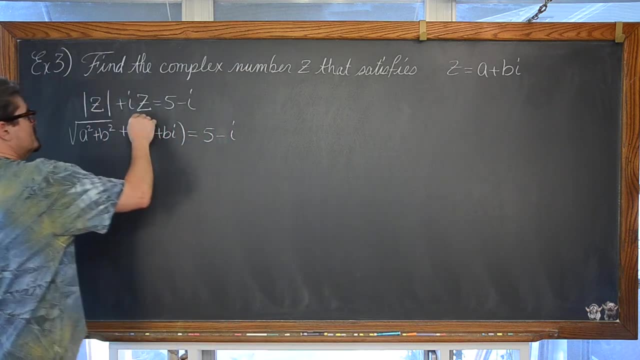 2, in earlier classes. if you solved equations with a radical, you would isolate that radical and then apply the inverse math operation, In this case square both sides of the equation. So we're going to distribute the i. We have the square root of a squared plus b squared. 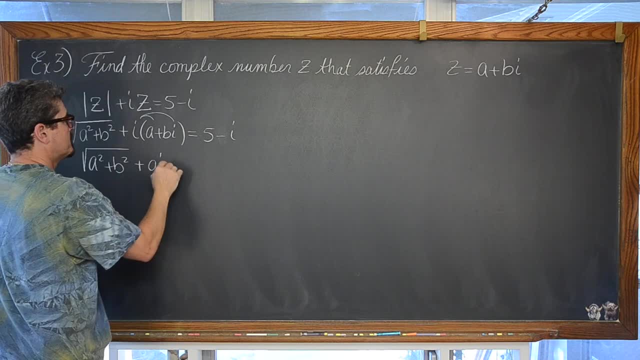 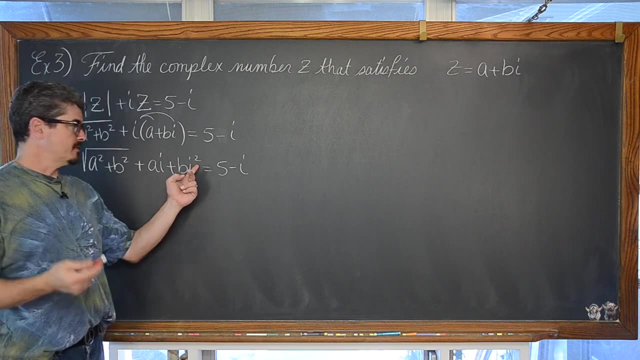 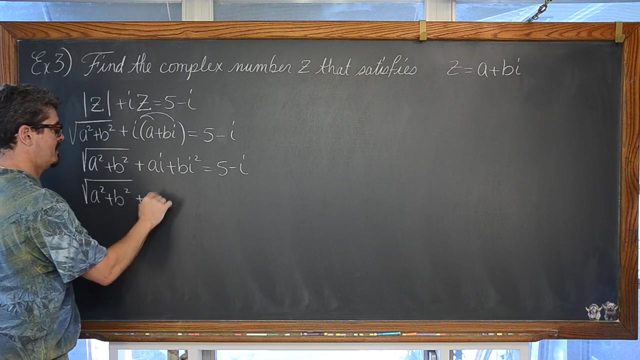 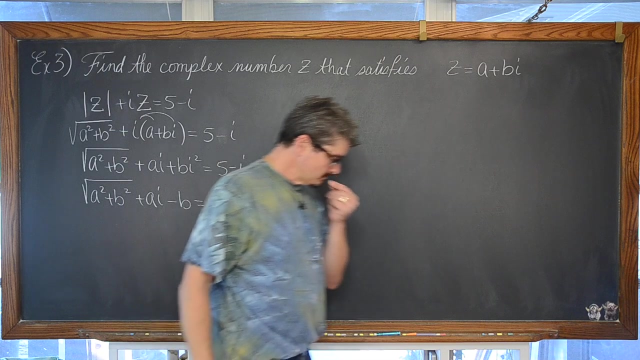 is going to be then added to ai plus bi squared equals 5 minus i. Well, let's not forget again that b squared is negative 1, so now we have the square root of a squared plus b squared. plus ai minus b, b squared is equal to 5 minus. i Seems like we're heading down a road here where we might 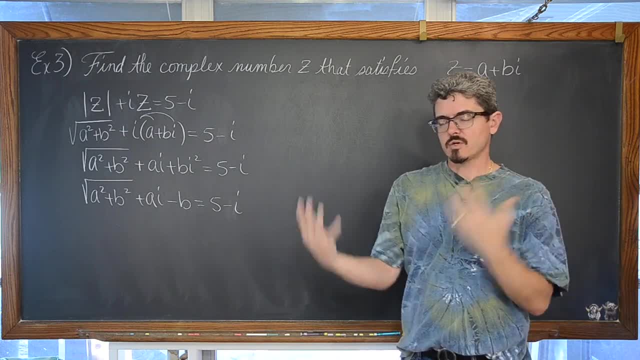 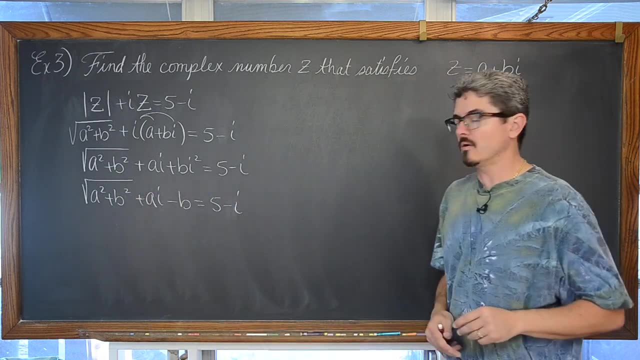 have that same situation where we're going to match up and compare the terms that do not have i in them and the terms that do, and maybe make a system of equations. So we're going to move everything away from our square root here And we have the square root of 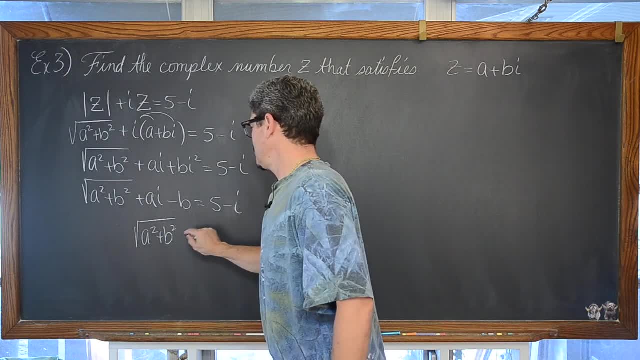 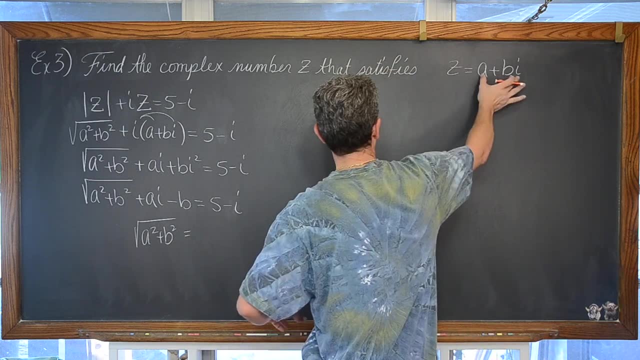 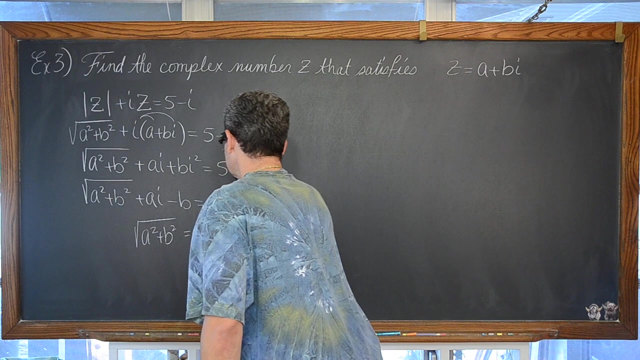 a squared plus b squared is equal to. Well, let's keep the terms without i together and the terms with i together, with this sort of like, again that real plus imaginary portion of our complex number. So we have 5 plus b and we have minus a, i minus i. 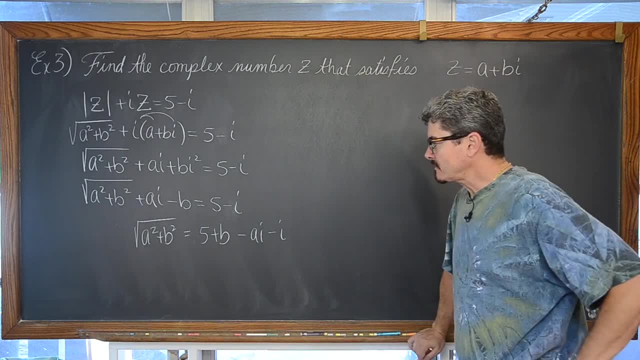 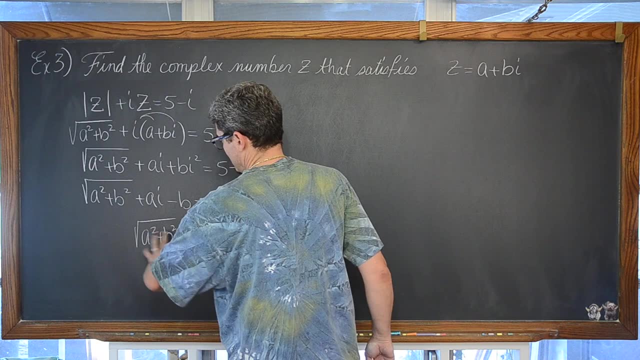 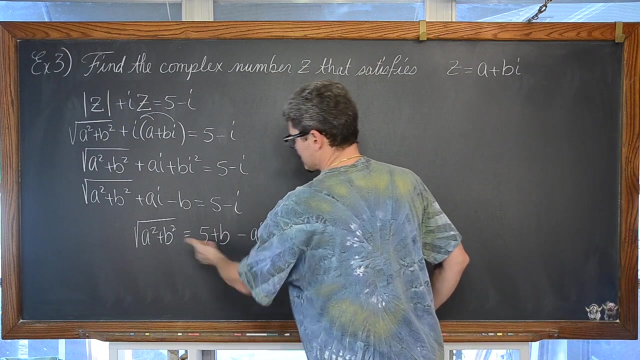 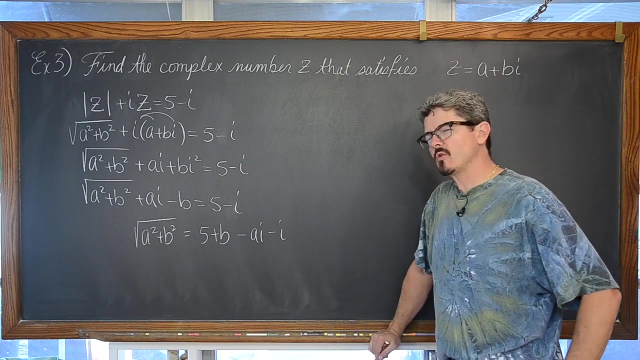 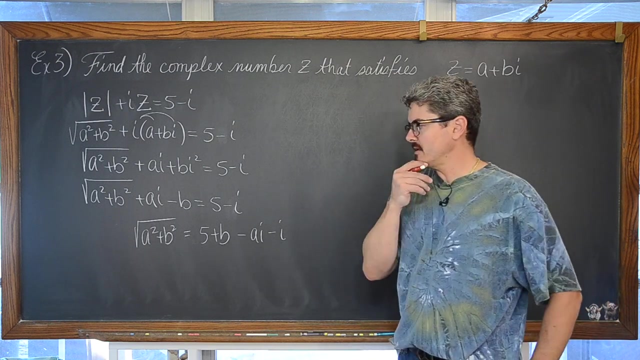 Okay, now, at this point you may want to take this equation and square both sides, but we're going to be squaring a four term expression which is going to probably become quite a mess. But if we write the right hand side of this equation in this real plus imaginary form, 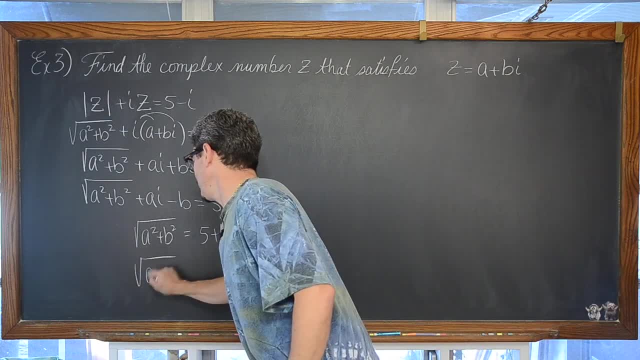 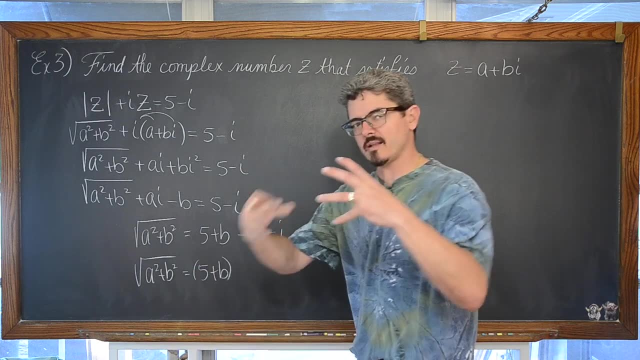 of a complex number. we have the square root of a squared plus b. squared is equal to 5 plus b. Already had that And I'm just going to put a parenthesis around this to highlight that that's like the two terms with no i's in it. 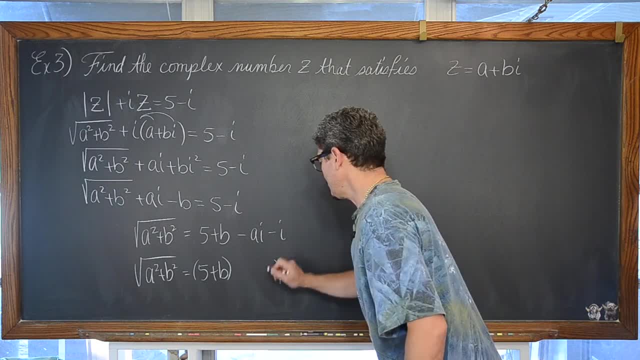 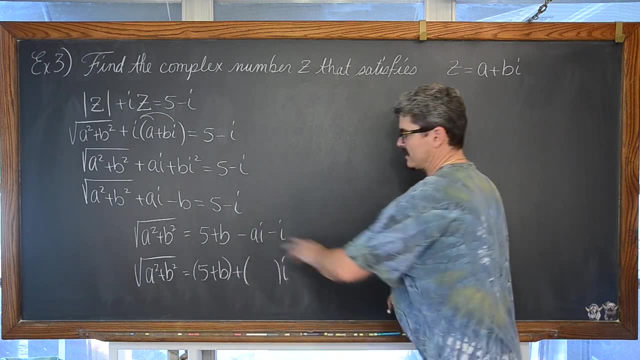 And we're going to factor out an i. I don't know why I just wrote t factor out an i That's going to give us and I'm going to write a plus sign here. so I don't have to worry about these signs, because I do want it sort of like an, a plus something. i. 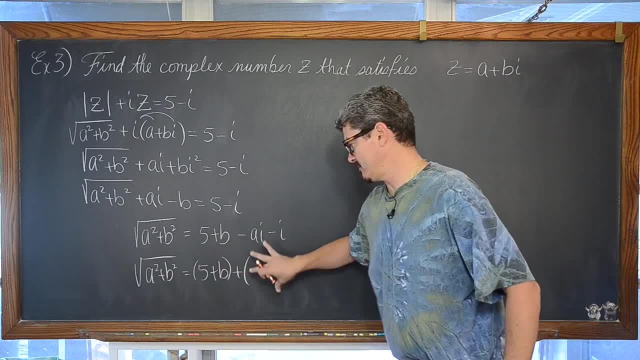 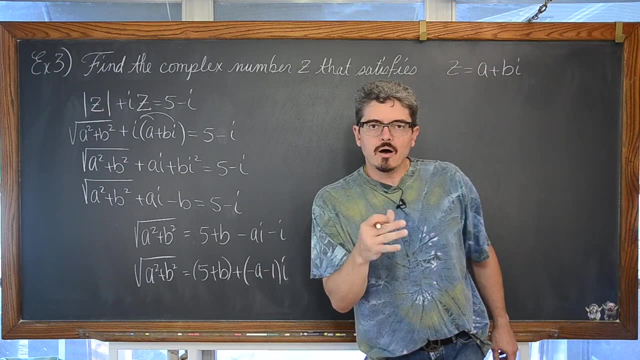 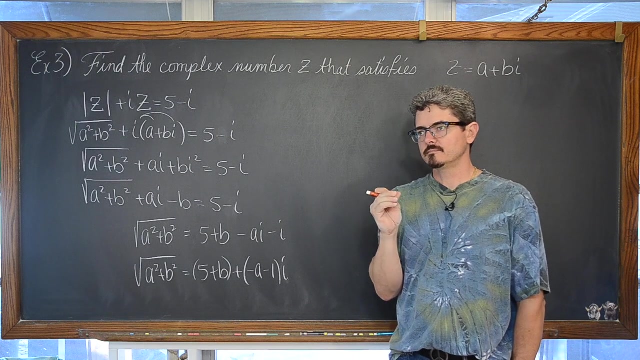 Well, not a, because that's going to be confusing because there's a here, but some real term plus some imaginary term of our complex number, negative a minus 1.. Now, the modulus of a complex number is the distance between the complex number and space. 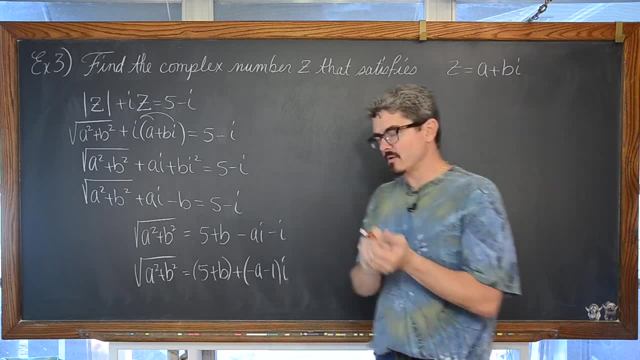 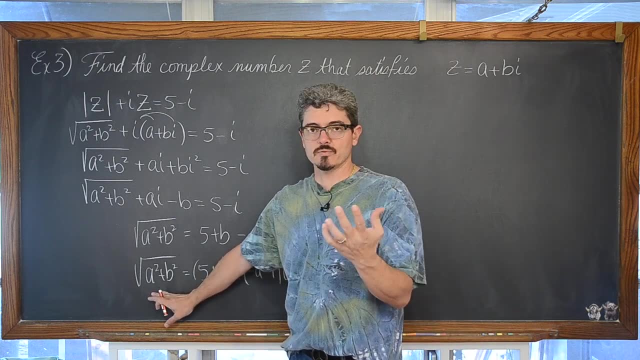 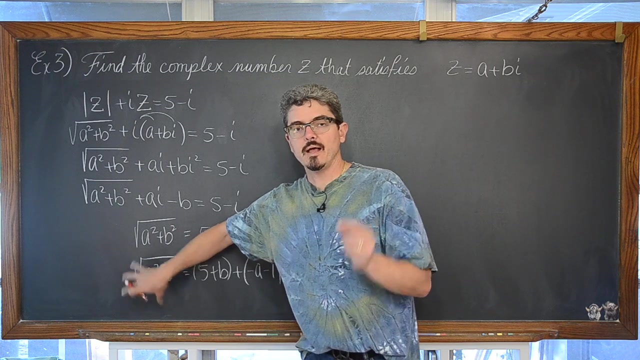 on the complex plane and sort of that origin or the center of that coordinate system, which means that this is a distance And distances have to be what Real numbers? So if the distance between the center of the complex plane and the complex coordinate has 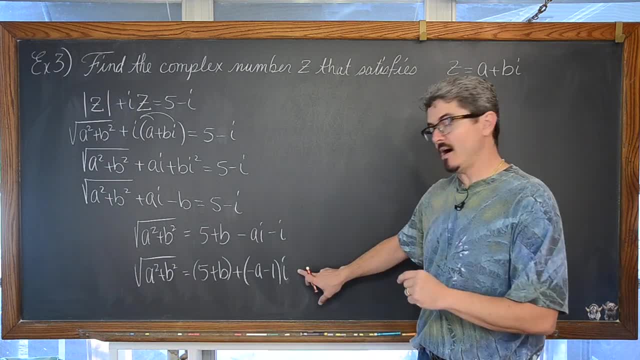 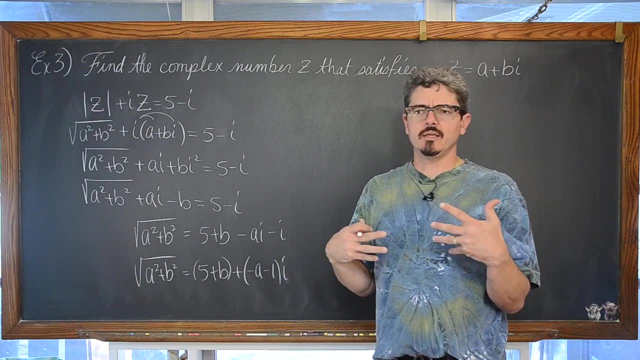 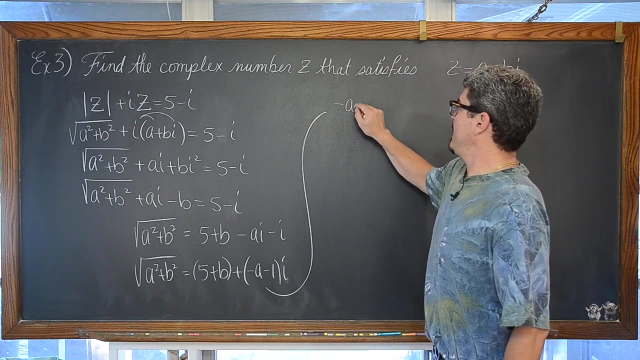 to be a real value, then the coefficient of i this has to be equal to zero, Otherwise you're leaving the door open to this modulus being basically a complex or an imaginary number. So, with that understanding, negative a minus 1 has to be equal to zero, which means that 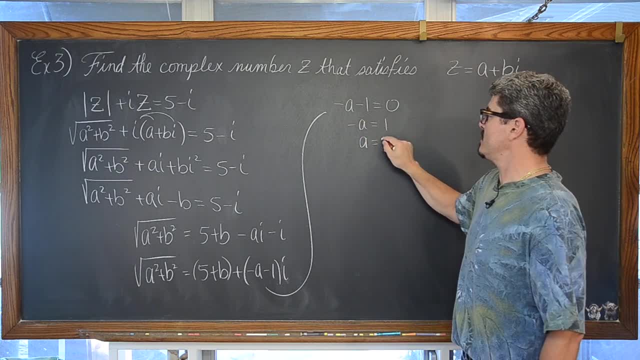 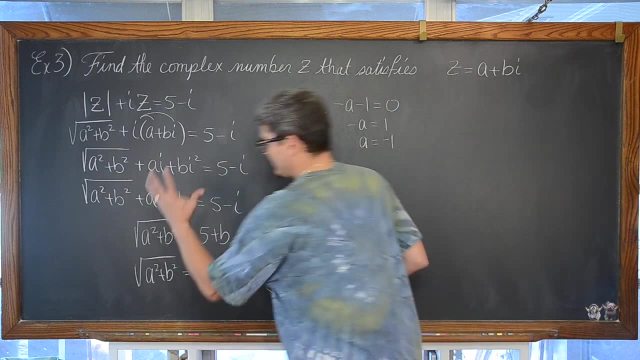 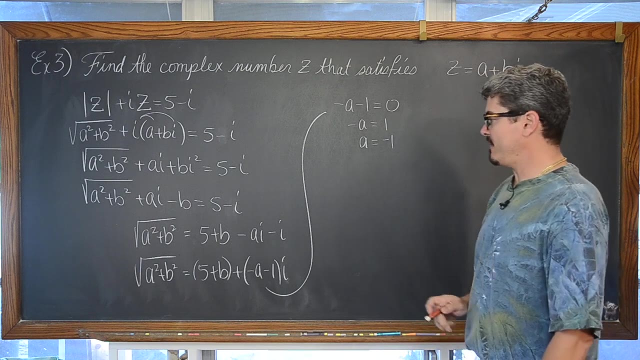 negative. a is equal to 1.. A has to be negative 1 for this coefficient of i to be zero, thus forcing this modulus of our complex number to be a real value. And now, using that fact, we have the square root. so, therefore, we have the square root. 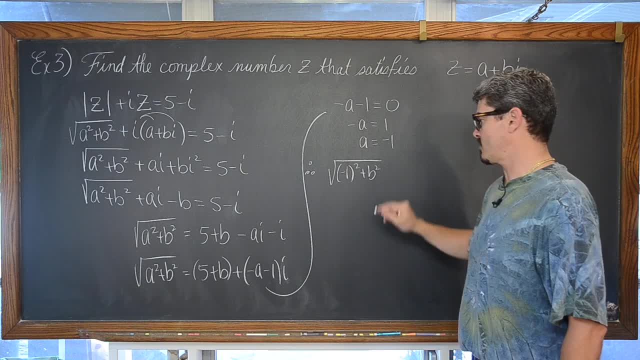 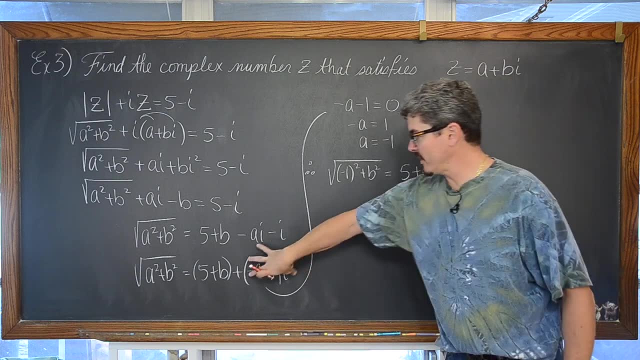 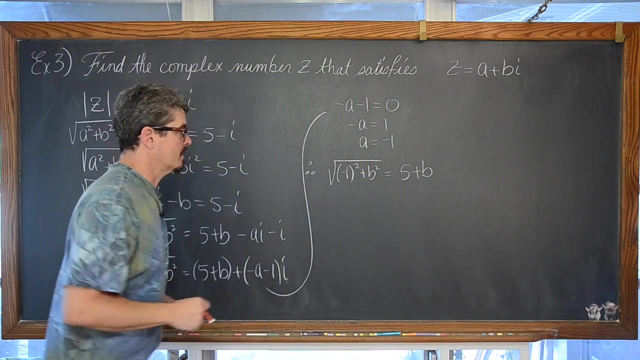 of negative 1, squared plus b. squared is equal to, well, 5 plus b. And we are setting, you know, we're making a equal to negative 1, we're forcing this imaginary term to be equal to zero again, for that modulus to be a real number. 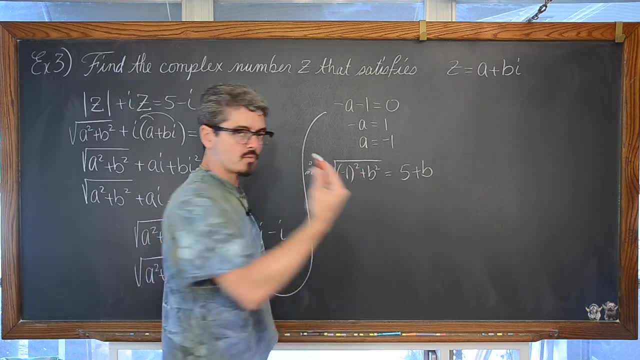 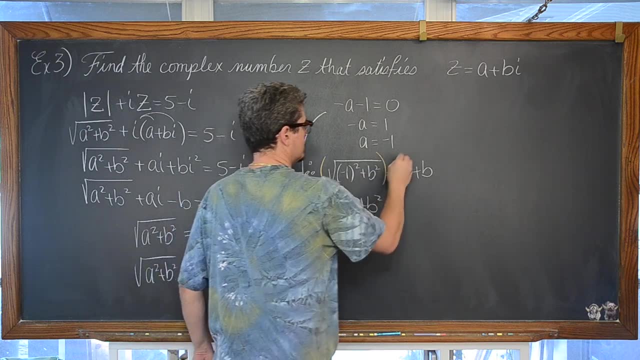 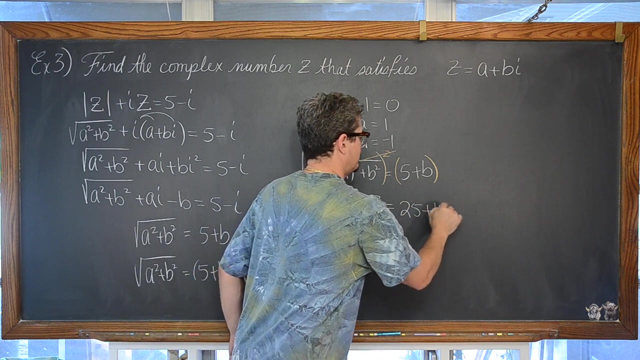 Now we're going to square both sides and we have: and negative 1 squared is 1, so we have 1 plus b squared and I guess I probably should show it squaring both sides. we have 25 plus 10b plus b squared. 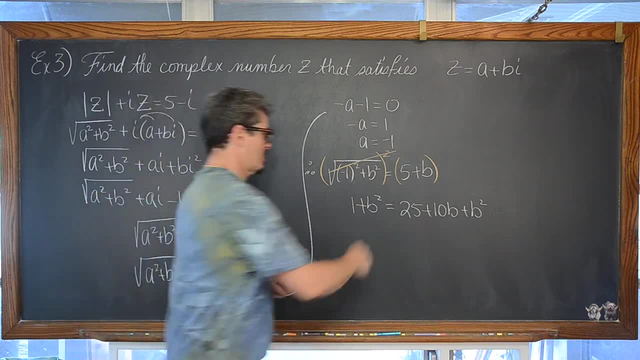 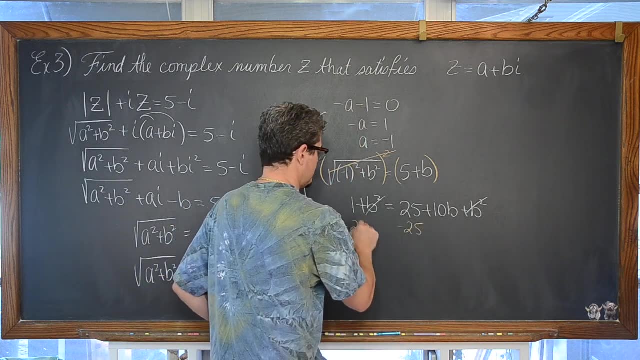 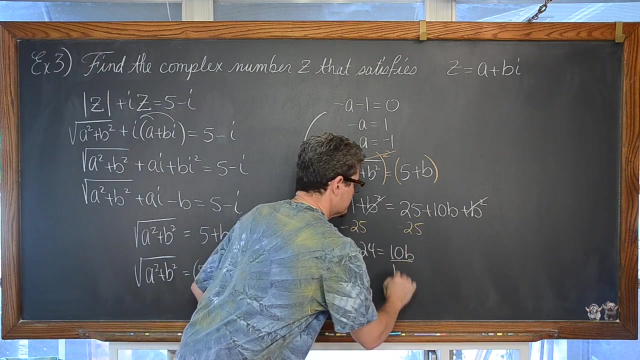 Okay, Both sides of our equation have b squared, subtracting that from both sides. And we're now going to subtract 25 from both sides of our equation And we have negative. 24 equals 10b dividing both sides by 10.. 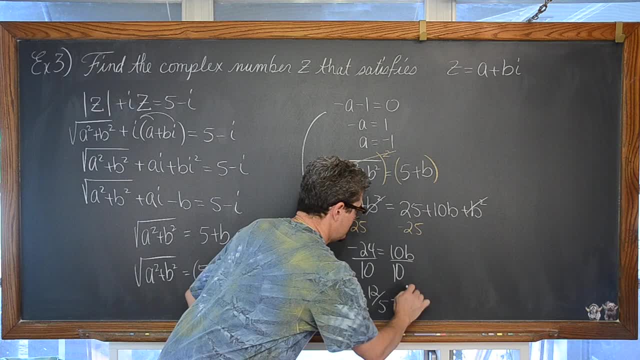 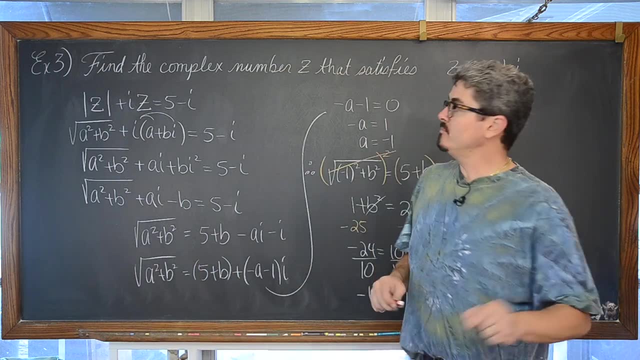 We have negative 12 fifths is equal to b. Now, before you celebrate, you are not asked to find the real values of a and b in this problem. You're asked to find the complex number z that satisfies this equation. so make sure. 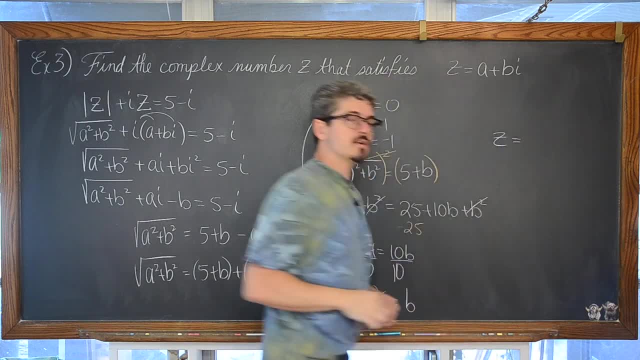 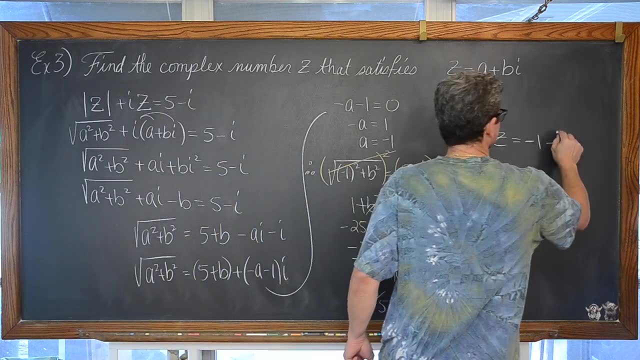 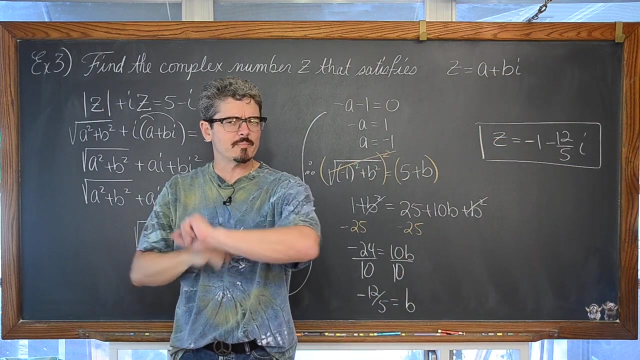 you format your answer correctly or that you actually answer the question. z is equal to negative 1, this is so exciting. minus 12 over 5, i- and that is the end of this example. I've got just one more coming up right now. 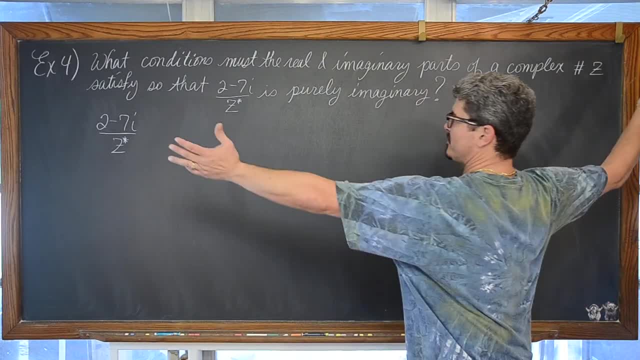 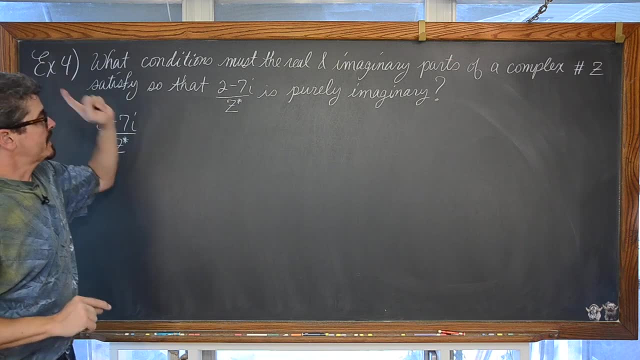 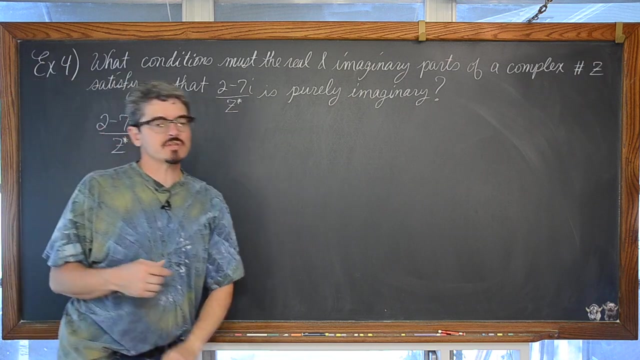 It's the last example. What, What conditions must the real and imaginary parts of a complex number z satisfy, so that 2 minus 7i over z star thingy is purely imaginary? Well, I don't know what notation your book is using, but hopefully it's the same. 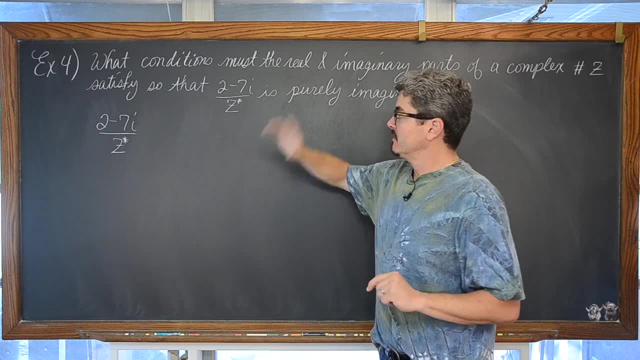 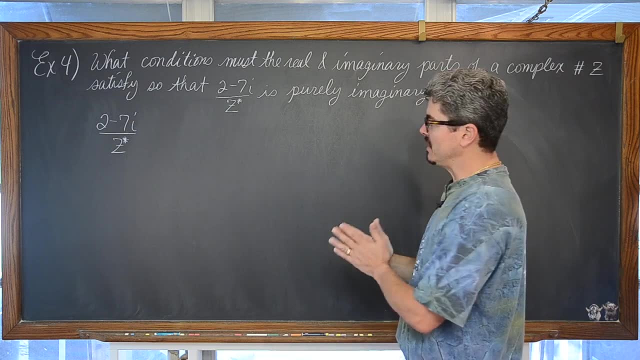 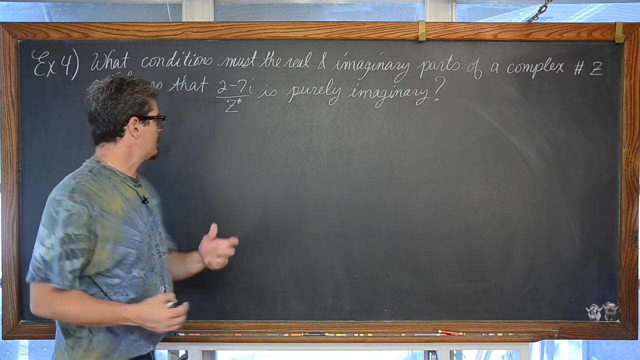 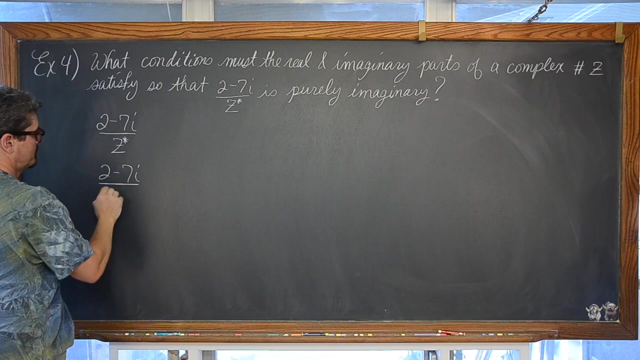 This represents conjugate in the book that I'm teaching from. So basically, we want 2 minus 7i divided by the conjugate of z, to be What? Purely imaginary. So instead of z being a plus bi, we're looking at z as being a minus bi. 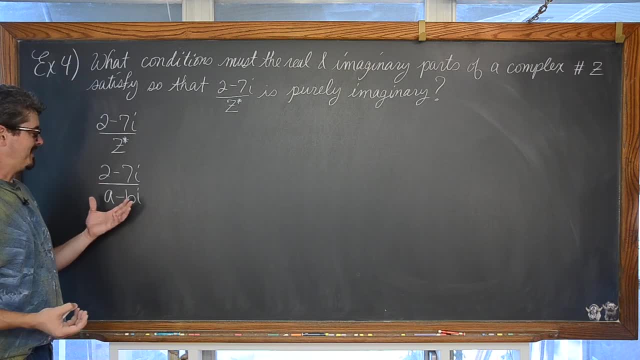 So, basically, we just need to rationalize, if you will, this complex fraction, get the i out of the denominator and then just figure out what needs to be going on with a or b or the combination of whatever, to make sure that this is purely imaginary. 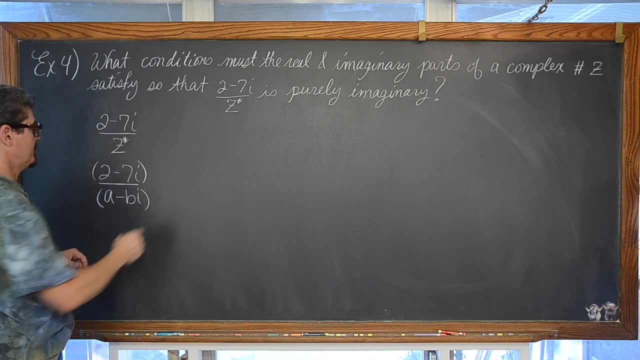 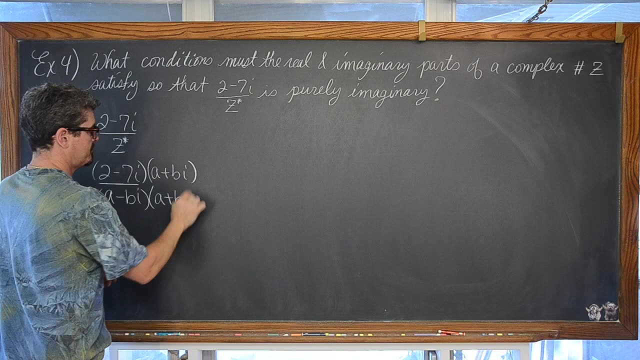 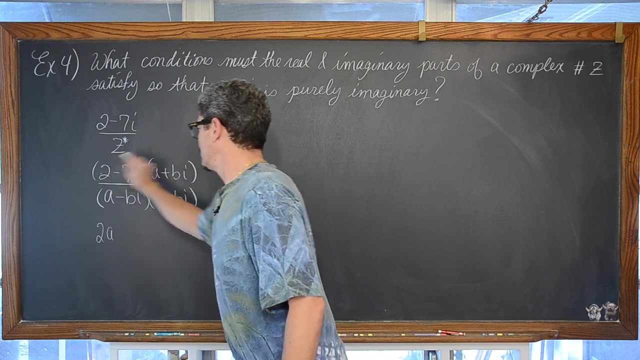 So we're going to multiply the numerator and denominator by the conjugate. So we're going to have a plus bi multiplied to the numerator and the denominator. That's going to give us 2 times a and 2 times bi. And now we have negative 7i over z star. 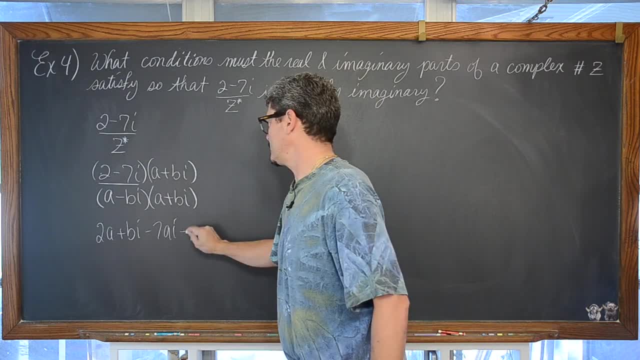 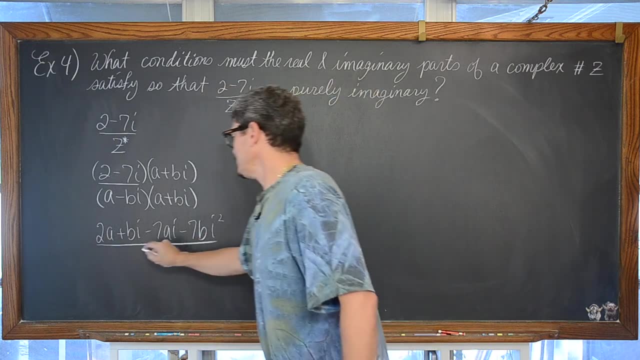 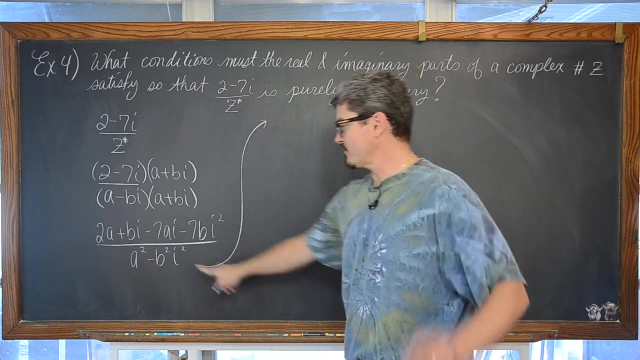 Okay, So that's going to be a plus a i and negative 7b, and then i times i is i squared all over a squared minus b squared- i squared. Okay. Well, don't forget right that i squared is equal to negative 1.. 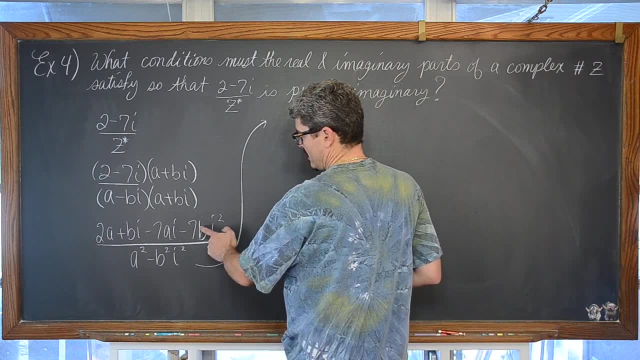 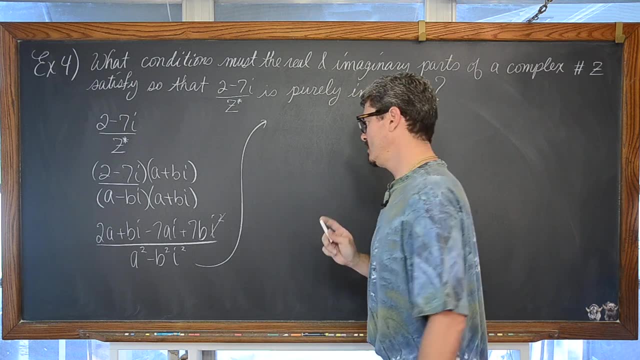 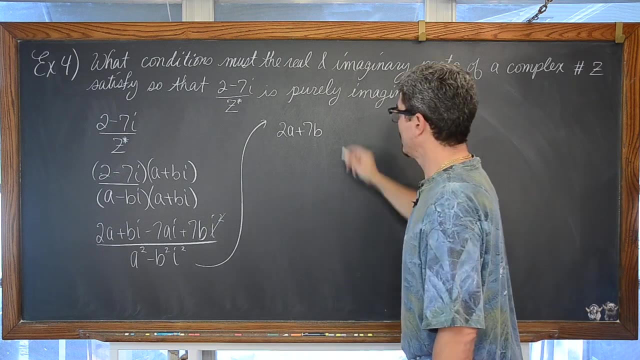 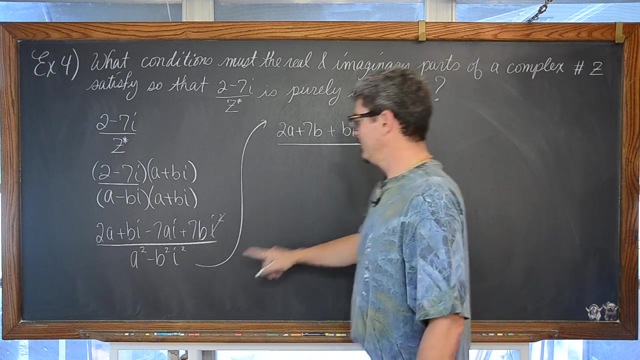 So we've got minus 7bi. squared is the same as plus 7i, So we're looking at 2a plus 7b. I'm putting these two terms together because they don't have a factor of i plus bi, minus 7ai. all over. well, again, with this i squared being. 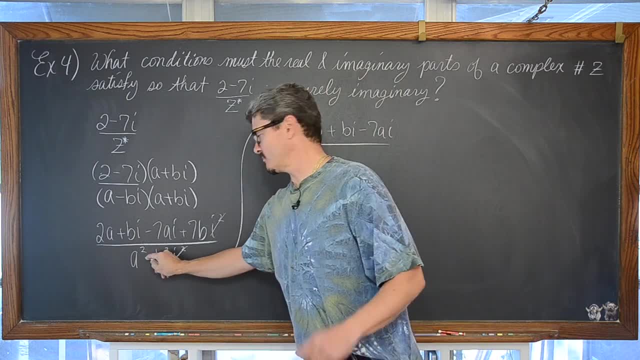 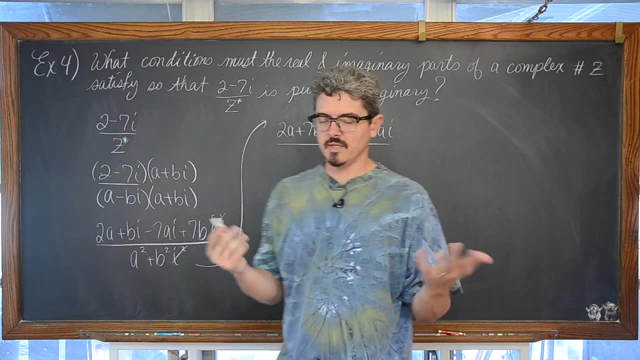 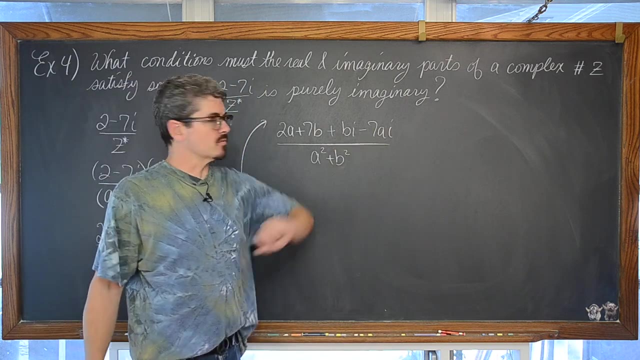 negative 1, negative 1 times b squared is negative. 1 times negative b squared is plus b squared, which a squared plus b squared is going to be a real value. Okay, So we're going to take out this factor of i and create a coefficient for the imaginary. 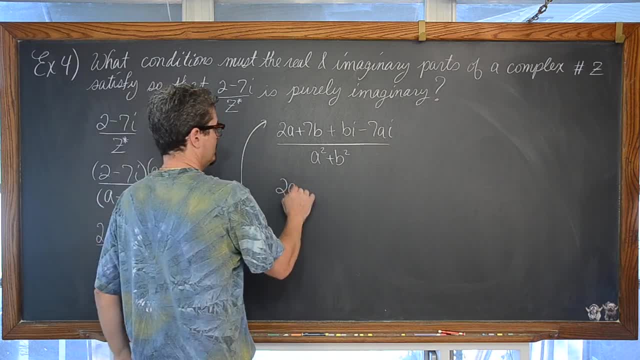 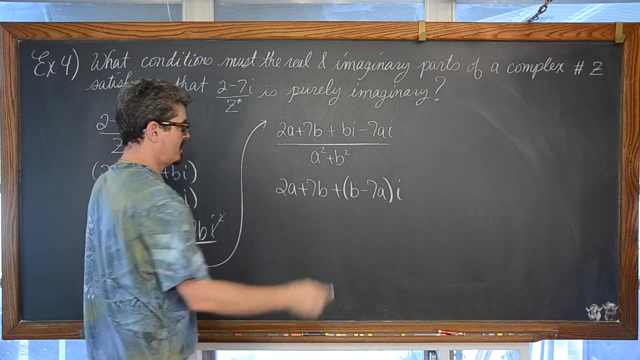 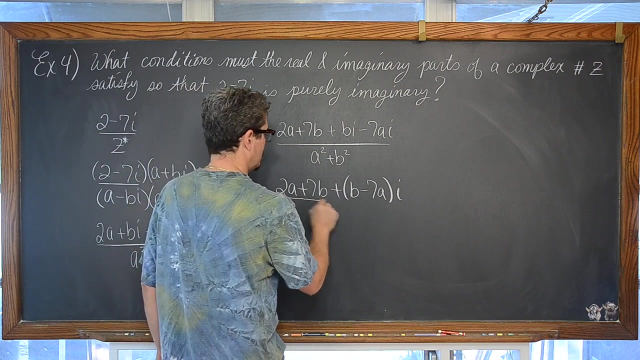 term of our complex number and we have 2a plus 7b plus b minus 7a, which is our coefficient of i, and I'm also going to actually separate this into two separate terms. where we have, this is over a squared plus b squared. 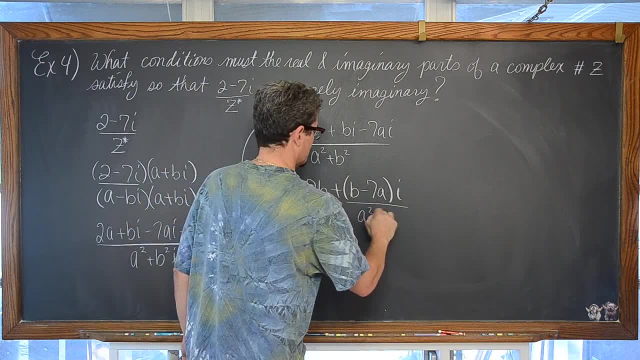 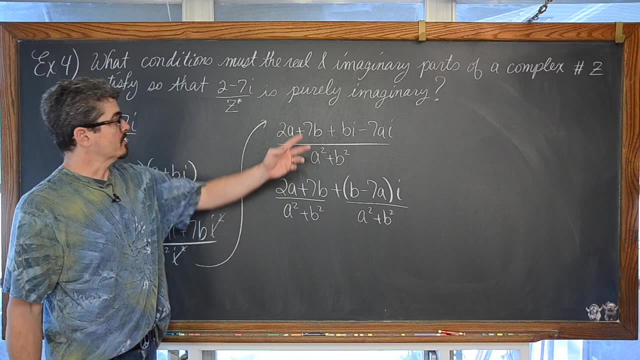 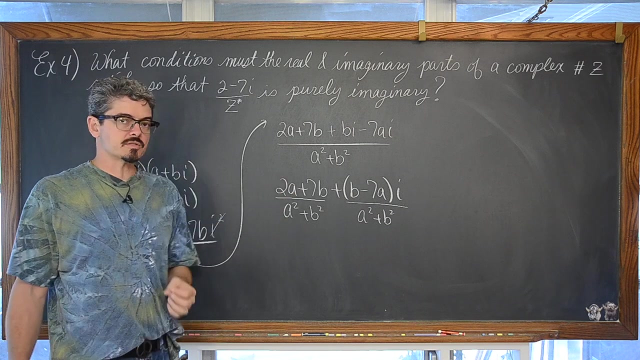 Okay, And this is again a squared plus b squared, which is going to be a real value. Now we want our complex number to be purely imaginary, which means that we want the real term to be equal to zero, And the only way you make a fraction equal to zero is if the numerator is equal to zero. 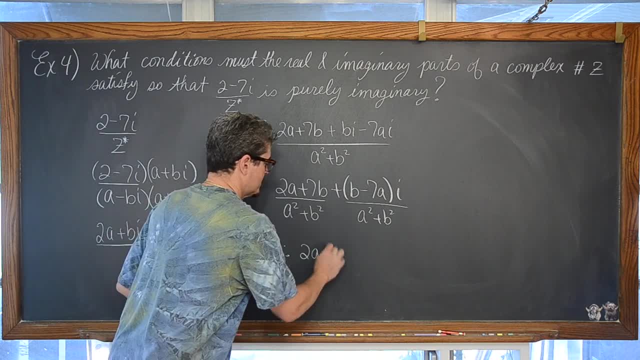 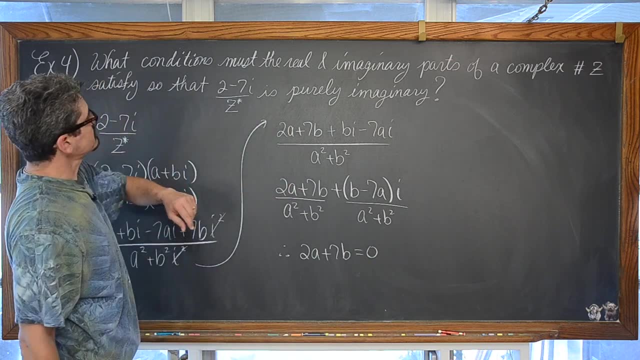 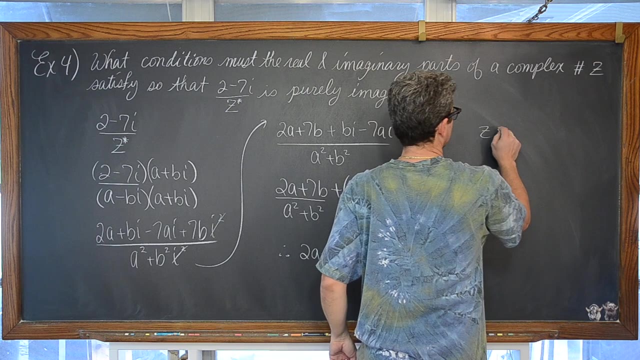 So therefore we have the 2a plus 7b has to be equal to zero And we're looking for The real and imaginary parts of a complex number z. So we are looking for some kind of complex number z and we're looking for the real and 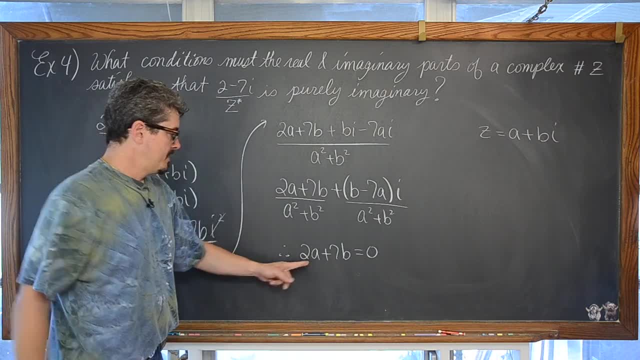 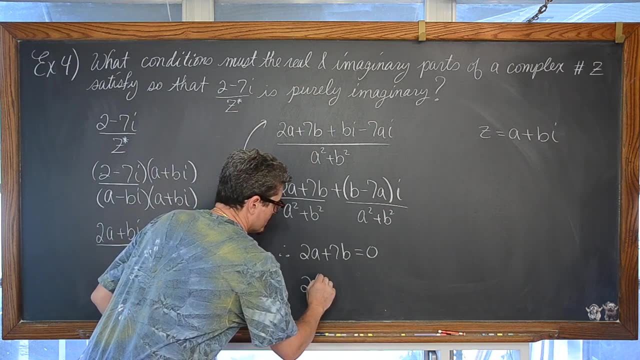 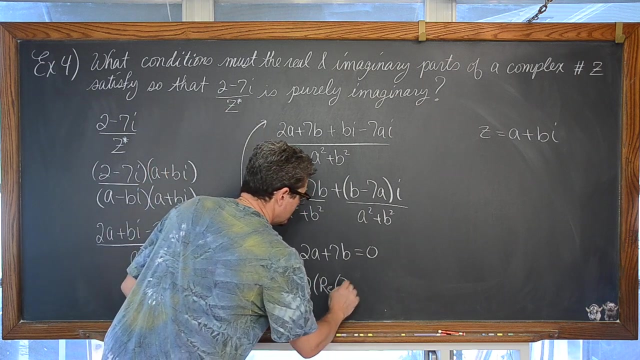 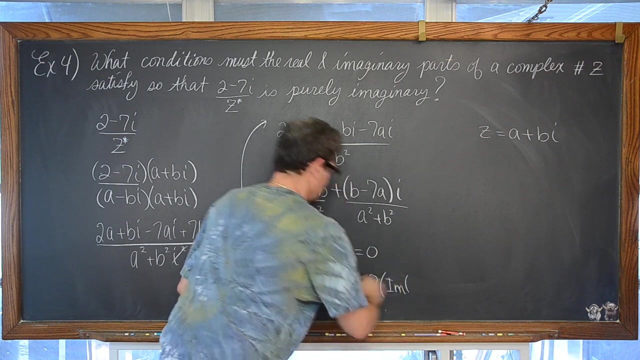 imaginary parts. So we have that 2, which a is the real part of this complex number. the 2 times the real portion- Make sure I use the right symbol here- The real portion of z. Okay, Okay, So the real portion of z plus 7 times the imaginary portion of z, which is a plus bi.